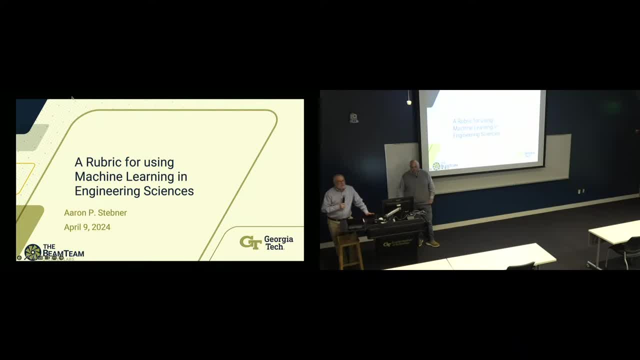 seminars. So it's a pleasure to have with us today for our final Nano at Tech for the spring semester- Professor Aaron Stebner. Aaron got his bachelor's and master's degrees in mechanical engineering from the University of Akron before getting a PhD, also mechanical. 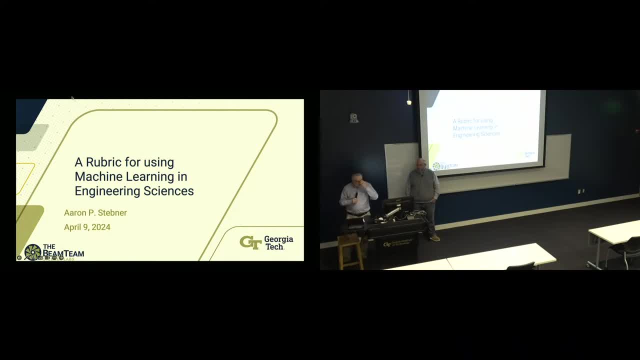 engineering at Northwestern and then doing some postdoctoral work at Caltech, And he's one of the rare individuals who's had experiences in government, industry and academia. I won't go through all of his career stops along the way, although I will say before we get to: 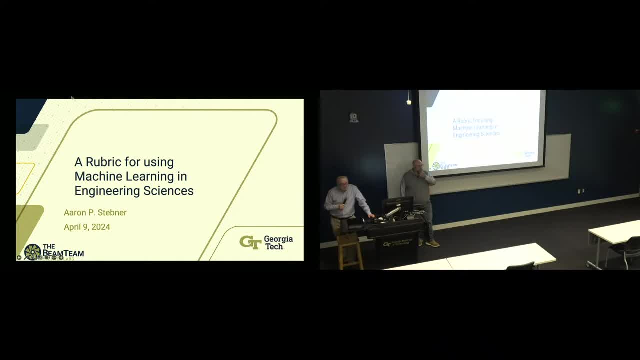 him. Before coming to Georgia Tech, he had a faculty position in mechanical engineering and material science at the Colorado School of Mines, where he was given the 2017 Researcher of the Year Award. He came to Georgia Tech in 2020, where he's currently an associate. 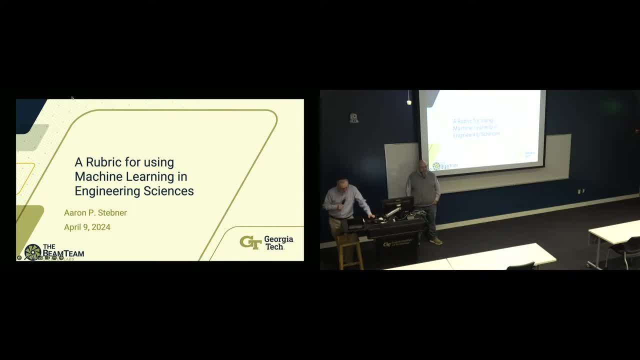 professor of mechanical engineering and material science and engineering and co-director of Georgia AIM and also associate editor of Additive Manufacturing. Thank you, And with that I will turn it over to Aaron. All right, Thanks, David, Great. So the talk today is going to be a talk on something that 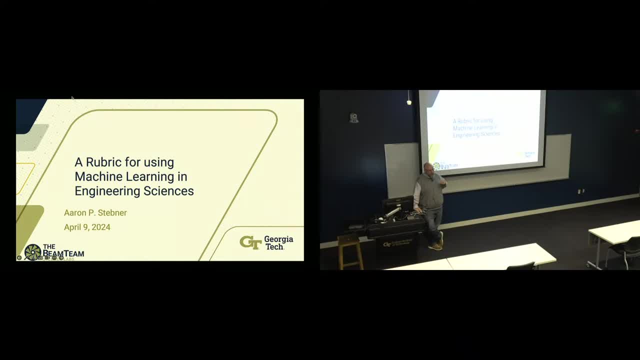 started as research activity in a center that I started in about 2015,, and then it's transitioned. You mentioned, a deputy editor for a journal has influenced a lot of this, and now this is also the basis for a course And I teach here at Georgia Tech, which next fall will become a permanent course and one 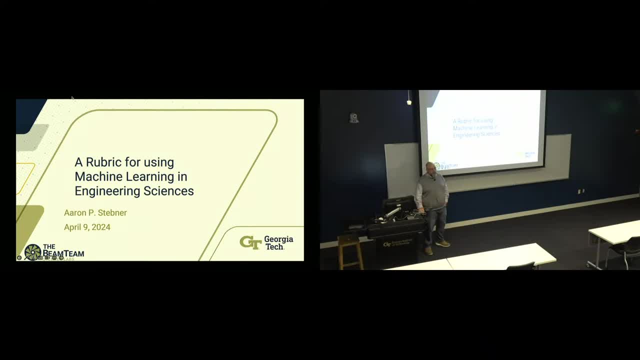 of the core courses for our new AI minors for undergraduates. So this is kind of an interesting activity for me over the last 10 or so years that has gone from being that kind of cutting edge research and now transitioning it into undergraduate education where I think machine. 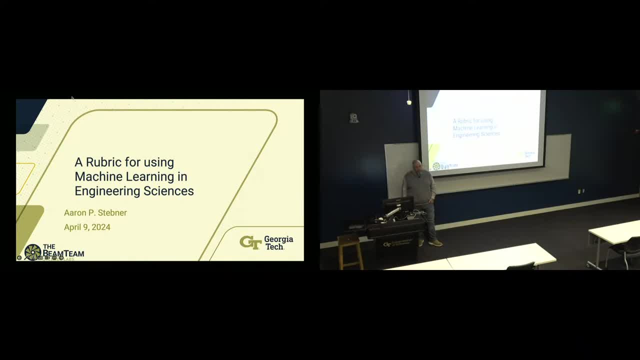 learning, especially as a tool in engineering, is going to be a very important part of our lives. So I think that engineering has now starting to become a prolific practice, right? It's no longer this niche like a few people work on it and understand it, but rather everybody is expected to be able to pick it up on a daily basis in their careers, at least for the generation of engineers we're producing now, right. 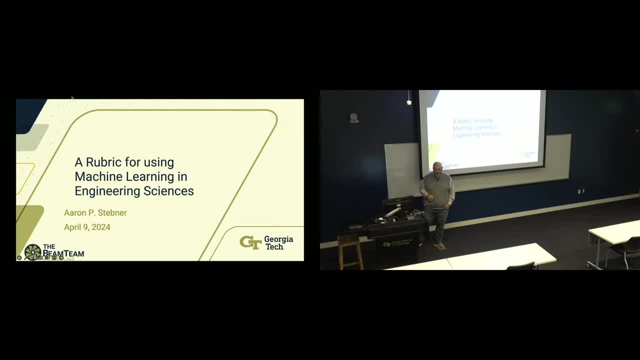 Maybe not us old guys, but maybe certainly all the younger folks in the room are going to be expected to be able to interact with and know and understand machine learning right, And so the work today is going to be largely at a high level. 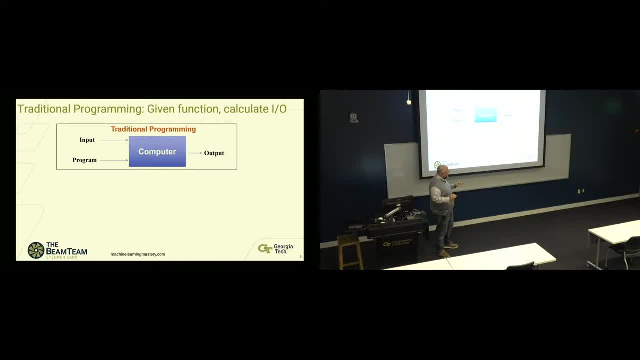 I think it's going to be a very important part of our lives. Thank you, Thank you, Thank you. I think it's going to be a high level, with some specific research examples thrown in to demonstrate what exactly do I mean by the different concepts. 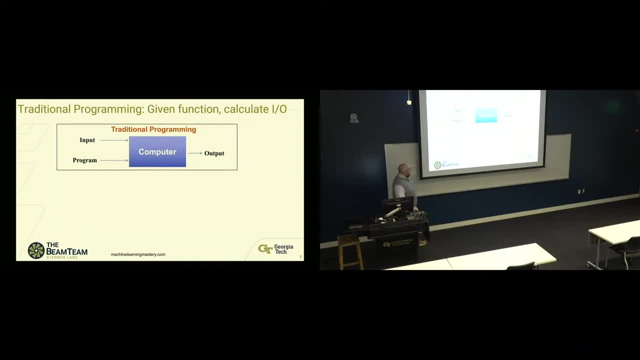 All right. So before we jump in, always good to start out with. okay, what do we mean when we say machine learning What is actually happening And make sure everybody's on that same page, And so traditional programming that we learn? my generation Eric can probably relate our handheld calculators. 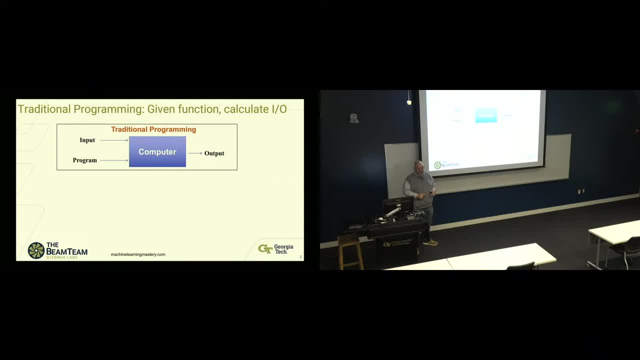 And being able to plot parabolic functions and things to help us in high school geometry and trigonometry right. we typically we know our inputs and we give the computer a program that we want it to calculate and the computer calculates the outputs, right? 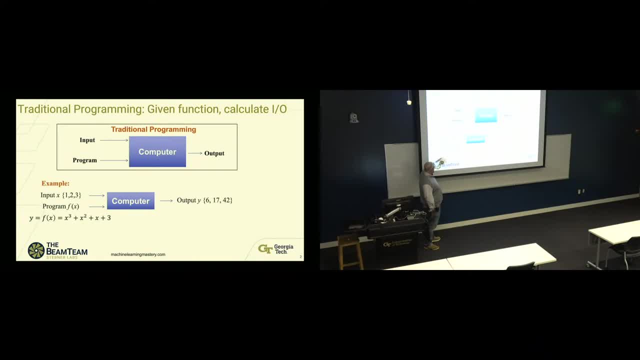 And so this is that example from high school math where, right, we write this program into the computer, we give it a set of inputs there and the computer calculates the outputs, And the computer tells us the outputs for that function are 6,, 17, and 42,, right. 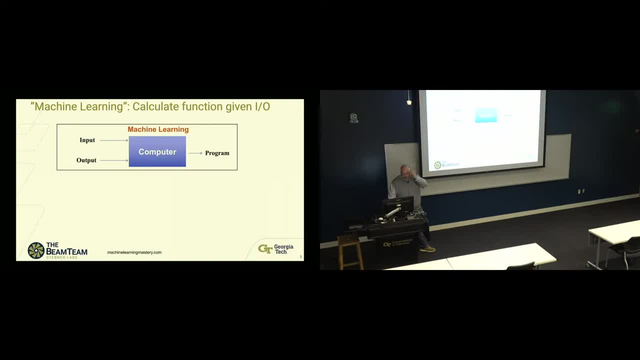 And what we do instead in machine learning is we know the inputs and outputs and we don't know the exact functional form, And so machine learning algorithms are all designed to figure out. if I'm given this set of inputs and outputs, what is the best functional form to fit my data. 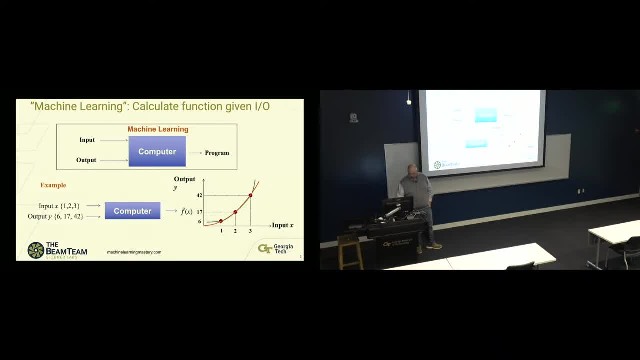 And the answer to best could depend on whether we want to do it in a more functional way. We want to interpolate or extrapolate or minimize variance- right? It depends on the question we're asking, And this is kind of where machine learning meets engineering science is. is that what it depends on? the engineers and scientists know, but the functional form and statistics are usually what the computer scientists or industrial engineers know, right? 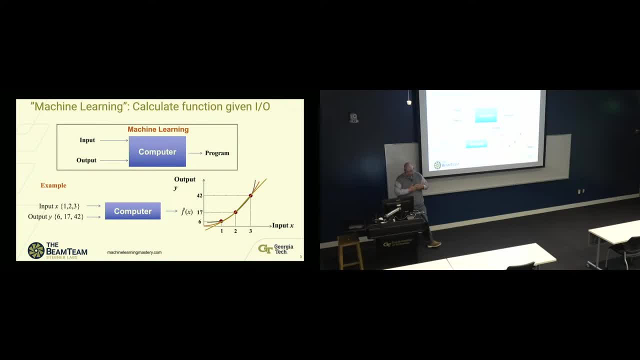 And so there has to be this kind of intersection to use machine learning and domain scientists to understand For my particular problem, am I trying to extrapolate? so I want the function that minimizes the variance outside of my data, even though it may not fit my data the best inside the window. 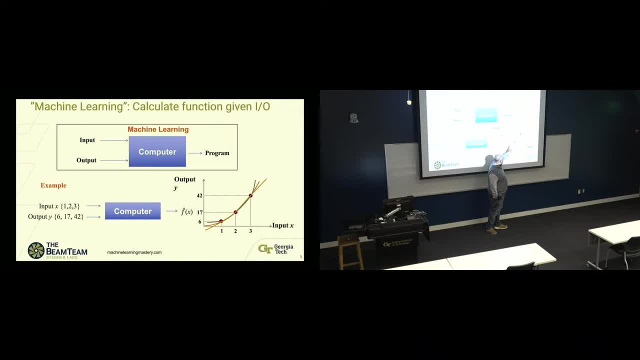 Or am I really going to interpolate and therefore I don't care that this one has these big tails that diverge, because it fits my data the best inside the window I care about, right? This is one example of where this machine learning needs to be able to meet the domain science, right? 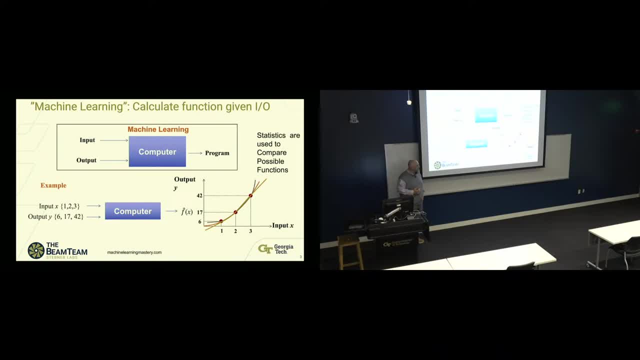 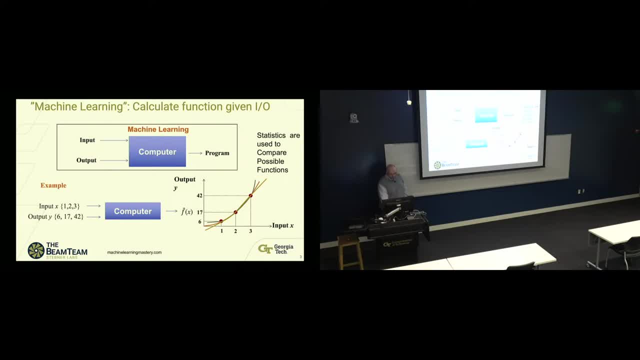 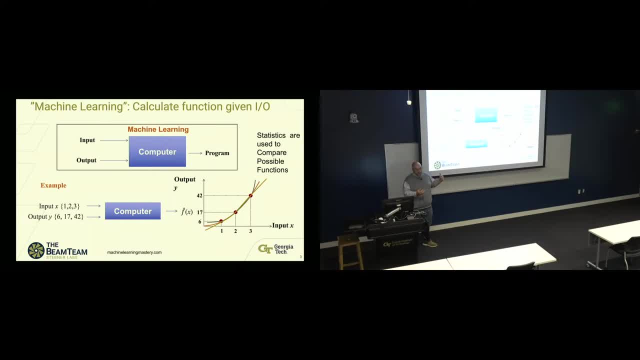 And in fact we're going to see as I go through the talk. really, machine learning is statistical modeling, just like Charles Fisher introduced to the world in the late 1800s, early 1900s, to fit data to the farmer's almanack to help farmers know what crop to plant in the next season. right, 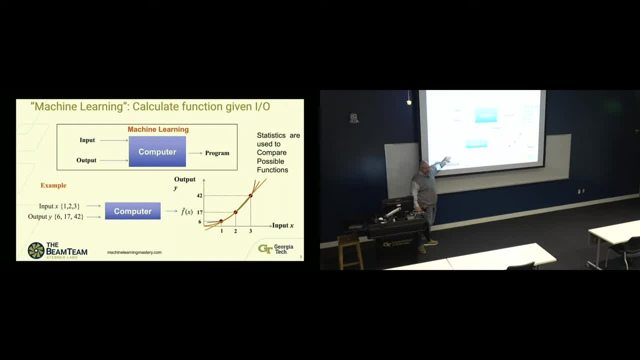 Just now we have computers that can do this in very high dimensions, higher dimensions than we could ever write down by hand on paper right. So now we can fit these statistical models and functions to our data in higher dimensions than we could calculate or work out by hand. and that's really the power. 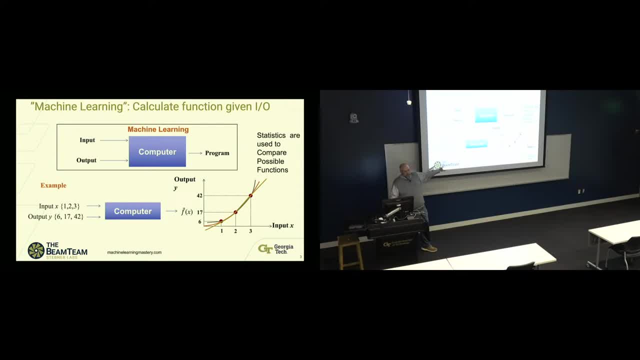 in machine learning and machine learning is learning, the best functional approximations to our data. So the coefficients, which we call weights in linear algebra right, and then the functional forms, or the set of basis functions that we're gonna fit the weights to to model our data. 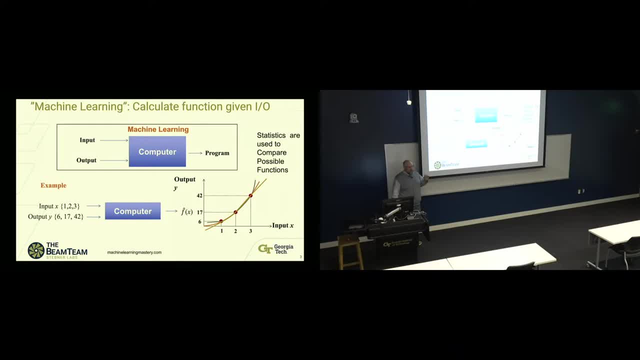 And so that really what the machine learns is the estimates and combinations of our basis functions and the weights of each of those basis functions in the model of our data, And so that's kind of the takeaway, but it can do it in many more degrees of freedom. 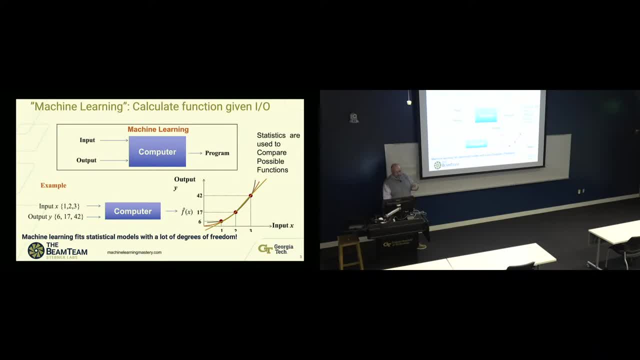 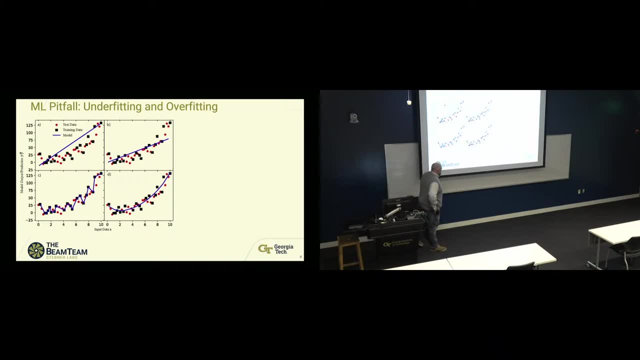 than we could ever program by hand. typically, or in fact, the algorithms that we do program for machine learning, work it out in arbitrary dimensions typically, And of course the pitfalls, or potential pitfalls, then become overfitting and underfitting our data. 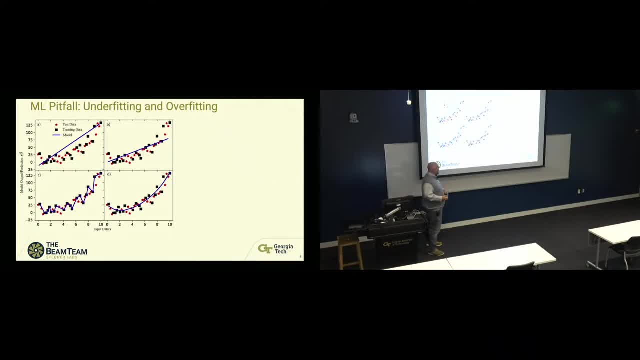 just like we may have learned in an undergraduate laboratory course in engineering. right? So you know the example here. right, the black data, or the data we're fitting the function to, the red stars, are the ones we're reserving, right? 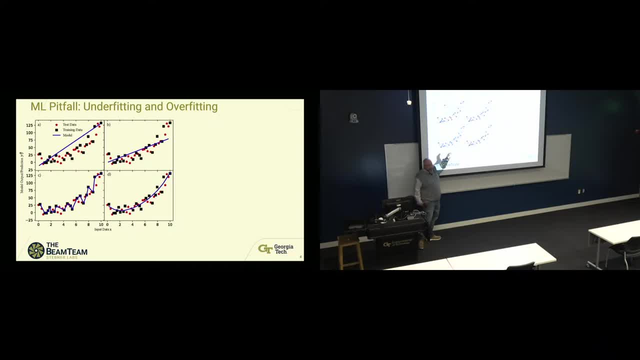 and if we don't have enough degrees of freedom, we get the upper left-hand corner where we're not modeling our data or our trend at all. so our model is not predictive for us versus if we put too many degrees of freedom. When I took a modeling class in graduate school, 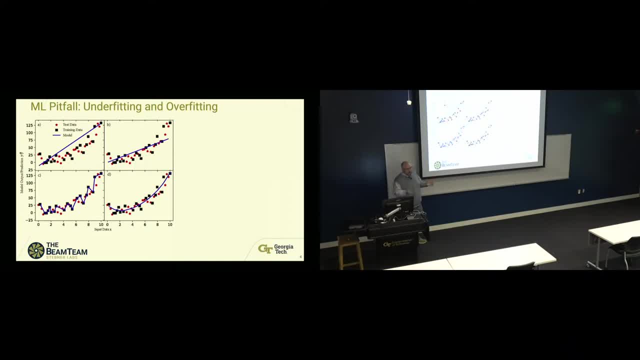 the instructor always said: you know, if you give me enough degrees of freedom in my expansion, I can model an elephant swinging its trunk to your line right. And so that's this case here where we can model every data point we're training exactly. 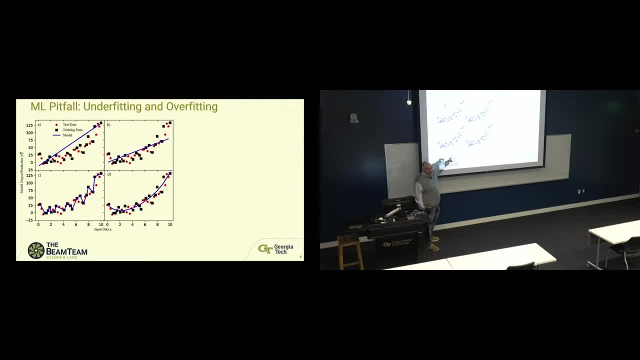 but then the minute we try to predict, we're complete garbage for the things we haven't trained on right. And so the art of you know really using machine learning for engineering sciences problems is understanding how to apply this picture to our engineering problem. 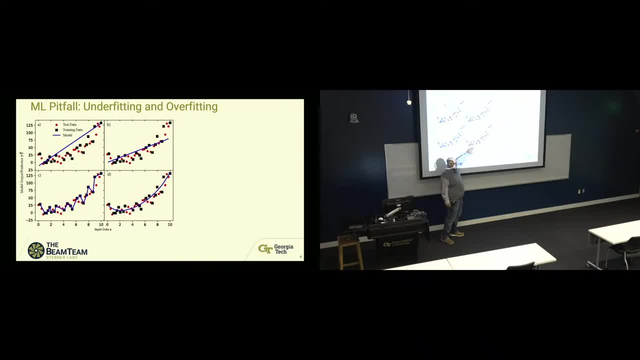 and know when we've hit this one as opposed to one of these other pictures. right, And that's really the challenge is this happens in higher dimensions than two dimensions, so a lot of times these simple plots or knowing how to reduce the question we're asking. 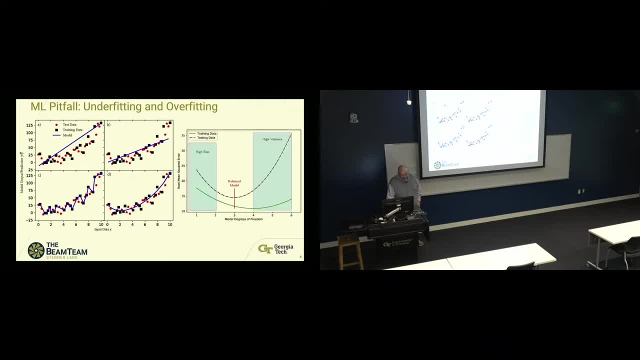 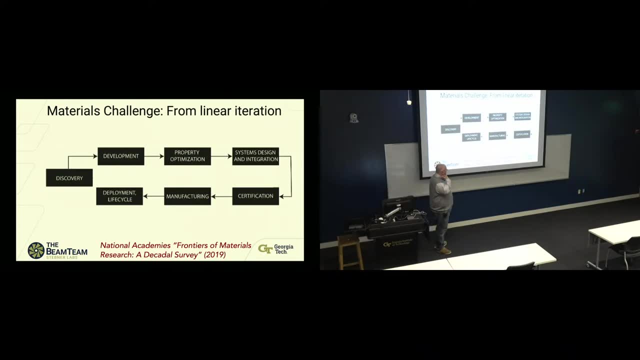 to these simple plots is where the expertise needs to come in. All right, And so why do we care about this right now as a nation? So this is every 10 years. the National Academies advises, you know, the National Academies advises. 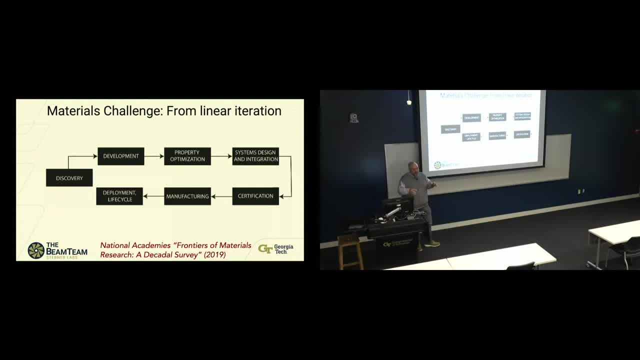 our politicians and government where our science and engineering investments should go for the next 10 years. They publish what are called these decadal studies. There's one on materials and manufacturing and the priority they have said we need to have as a nation. 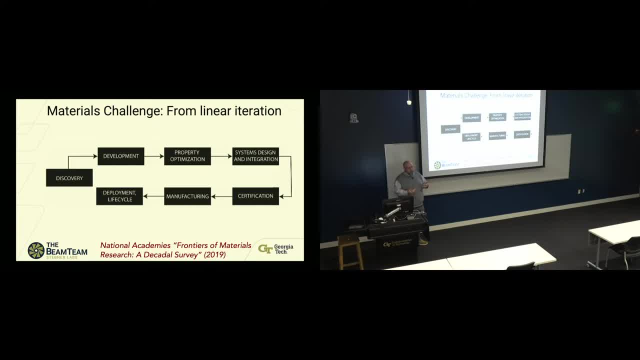 to maintain global leadership and, in fact, retain, get back into global leadership in some positions. as is a country, we need to move from the picture of discoveries happening in laboratories at universities to deployments in industry. being these long, linear, iterative loops, 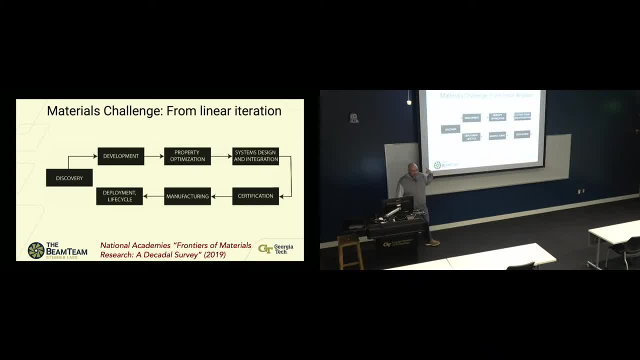 that often take eight or 10 years per piece if you're in aerospace, or two to four years per piece if you're in a medical device industry, for example, And we need to be able to instead design in all these stages at the same time, right? 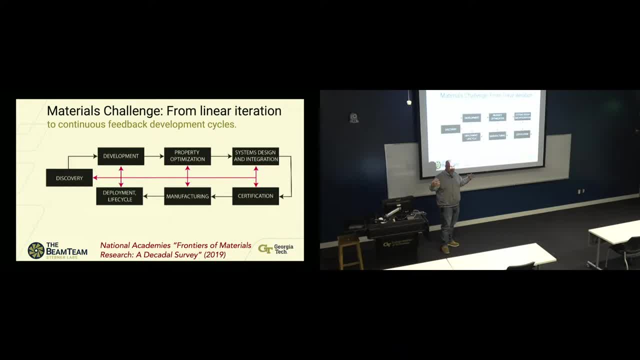 And really work on all of these in parallel and have them be interactive. That's the way to bring our time and costs down for getting new technologies out there. But of course this means we have to be able to consider all the degrees of freedom in each of these boxes. 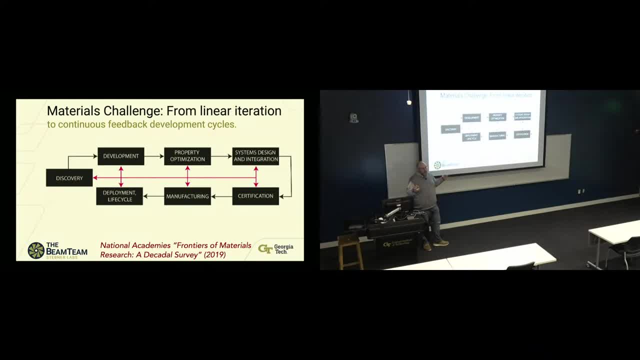 at the same time. and that gets us to this machine learning place, right? Because now we have more degrees of freedom and, in fact, more domains involved at the same time than any one person can work out, And so we need this statistical guidance. 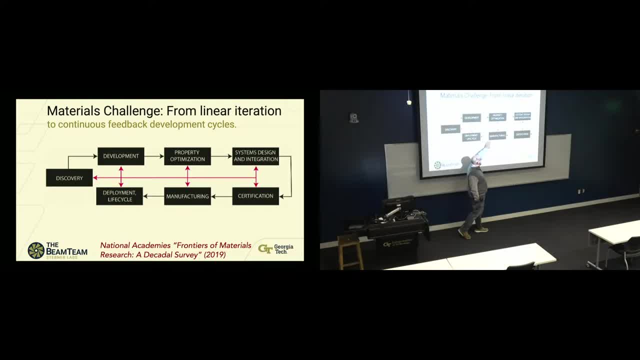 on, how should I be turning a knob in my manufacturing process or back here in my material discovery or material design process? right, And all these kinds of questions we need to answer that are typically done by large groups of people. 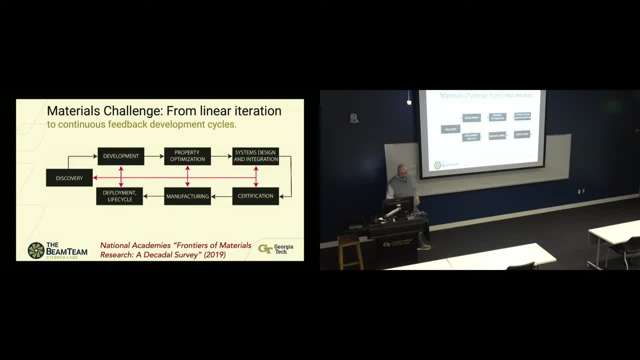 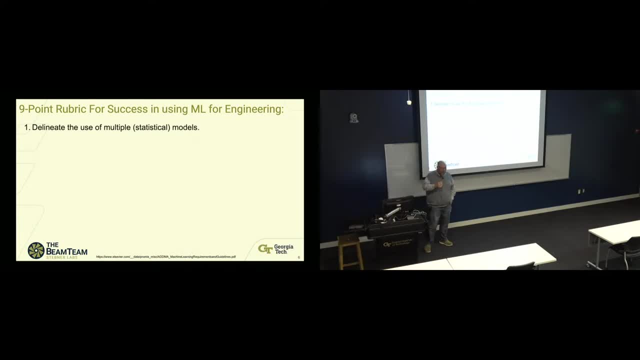 statistics and AI can help us get to this place where we can turn all these knobs at the same time. Okay, and so my takeaway out of all of this, over working on this problem, as it's been called machine learning for the last 10 years. 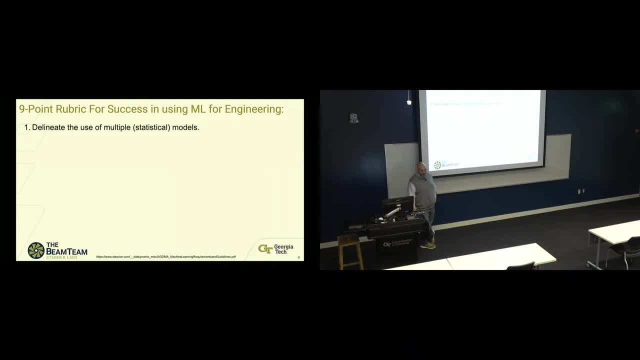 but really since the 1990s when I started in automation for manufacturing, is that machine learning, just like finite element modeling or density, functional theory or any of these other modeling tools that we have in engineering sciences, is not the right tool for every engineering sciences problem? 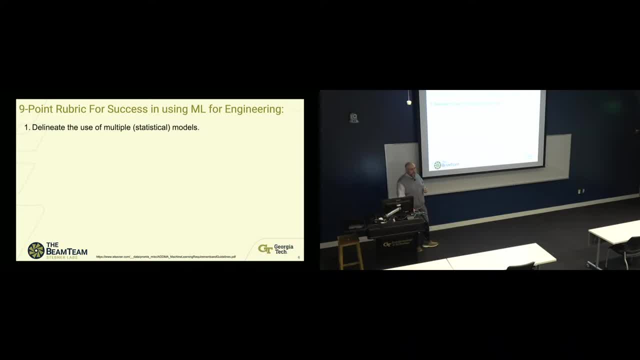 even if it involves data, And I'm gonna show some examples of that. So I know, 10 years ago, when I would hire a graduate student and we were just getting into this space, they would interview and they'd say: I wanna do a thesis on machine learning and 3D printing. 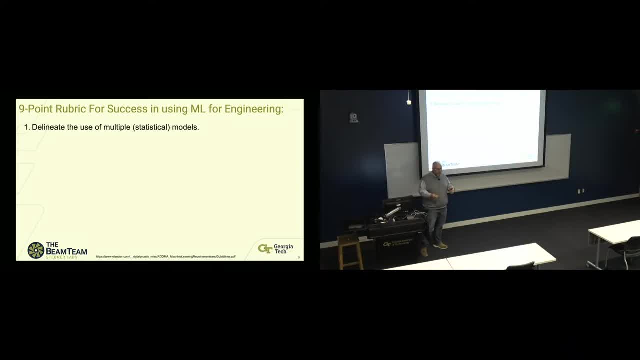 That's why every student was coming to my lab And I would say, well, that's good, but what problem are you gonna solve? Because machine learning might not be the right tool for that problem And I think we really need to realize. 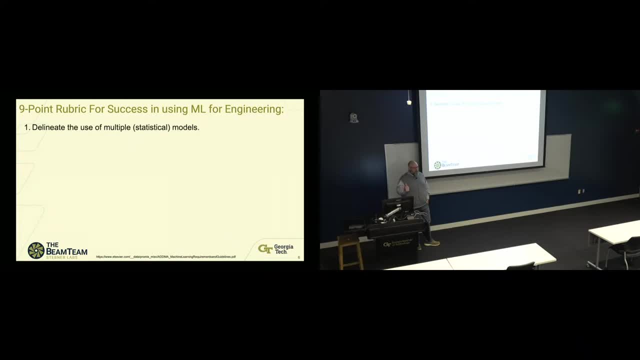 in applying machine learning in engineering sciences. machine learning is not always the right tool, so we shouldn't start out assuming the machine can learn it for us. right? We have to still know what question we're answering and what are the fundamental properties of the data. 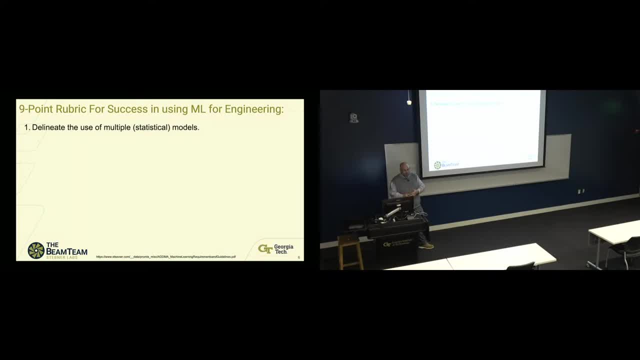 that we need to aggregate or model to answer that question, and then is machine learning the right tool. So the rubric really starts out, and so the rubric that I'm gonna show here today is actually part of the author guide for the additive manufacturing journal. 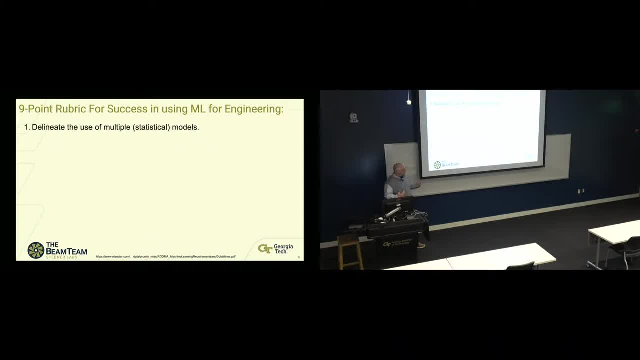 where I was deputy editor and we had to solve a problem where we were getting papers published that we knew were complete crap- in machine learning, to be honest- and then other papers that were really good were getting rejected, often after three, four, five rounds of revision. 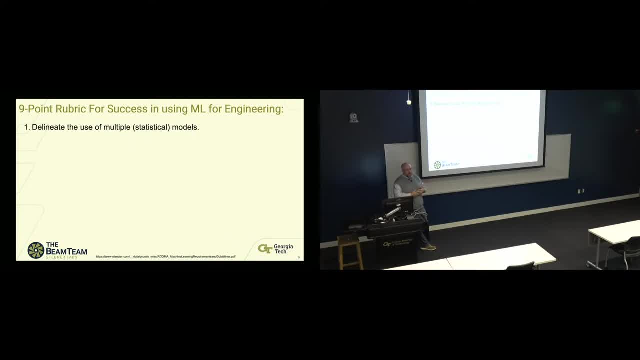 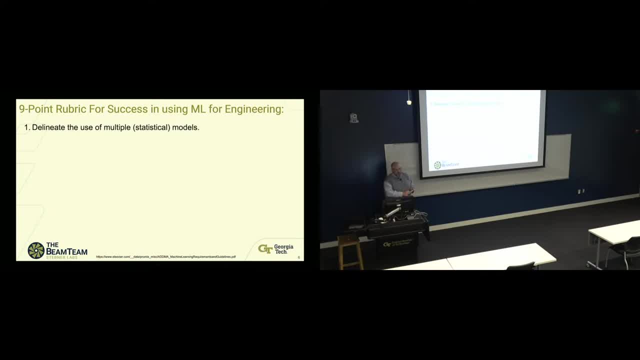 anybody that works in that space today knows: hey, I need to publish my input file. I need to talk about my energy minimization, whatever right we're in finite element studies, we have to publish our mesh refinement study, what kind of elements we use. 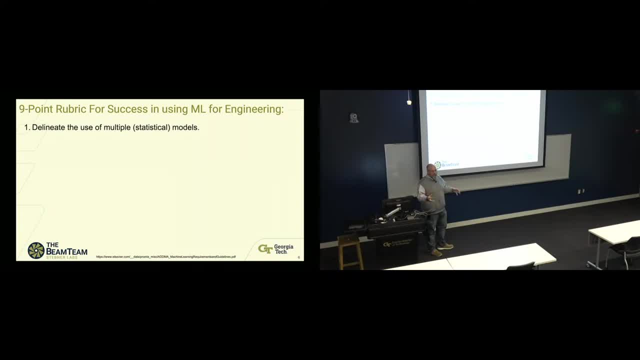 did we use nonlinear elements right? all these kinds of things that have become standards for working with other modeling tools. We needed standards for working with machine learning as a modeling tool in engineering, at least in our journal, so that reviewers could all uphold the same standard. 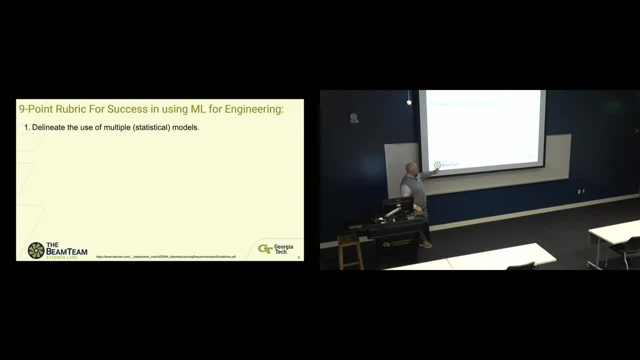 and know what the standard was for publication in the journal, and now these have turned into the basis for a class which I see a couple students who have suffered through the class sitting in the audience. but really we have a class where we now at Georgia Tech, where the first half 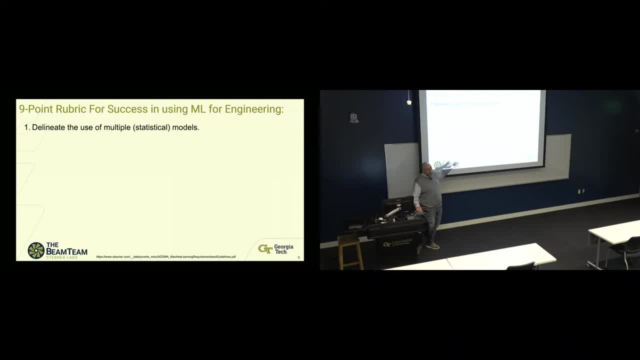 is kind of fundamentals, but then the second half is all case studies working through this rubric and different engineering problems in material science, mechanical engineering, chemistry et cetera. The first thing we need to know is: why are we gonna use the machine learning model? 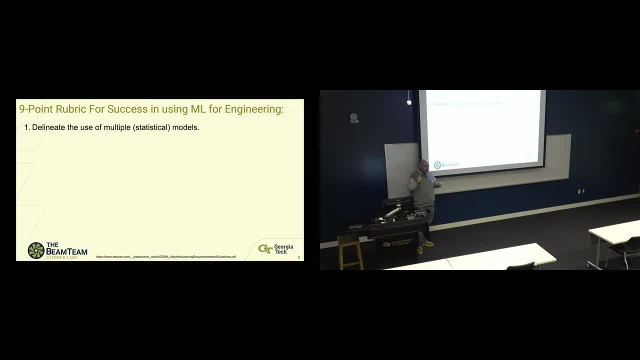 And often when we're using machine learning, we're not just making one machine learning model, but we're gonna make multiple machine learning models. We may have one model that says which of I may have 54 inputs in my data set. 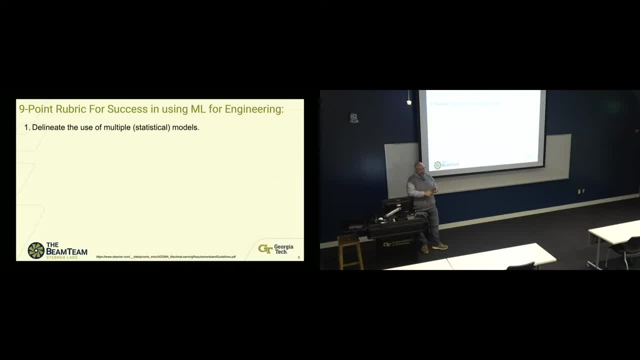 for example, if I'm working with materials, I might have atomic number, atomic weight, right, the composition of the elements that I put together and their stoichiometry, And we can go on and on and on: valence, electrons, et cetera. 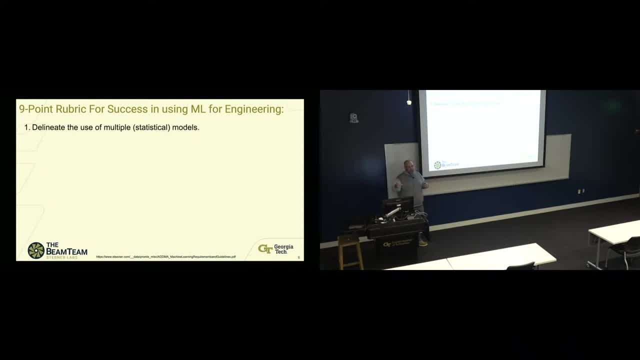 etc. which ones of these are most important to the question I'm trying to answer? If I'm trying to maximize the strength of the material, that might be a different set of features than if I'm trying to maximize the electrical conductivity, for example, And often we run. 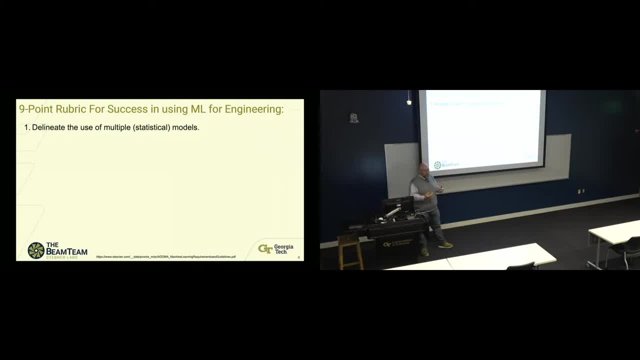 what's called a screening model or a feature importance model, before we actually build the machine learning model to help us with the alloy design. We want to reduce the number of features we have, And so usually when we're doing statistical modeling or machine learning, 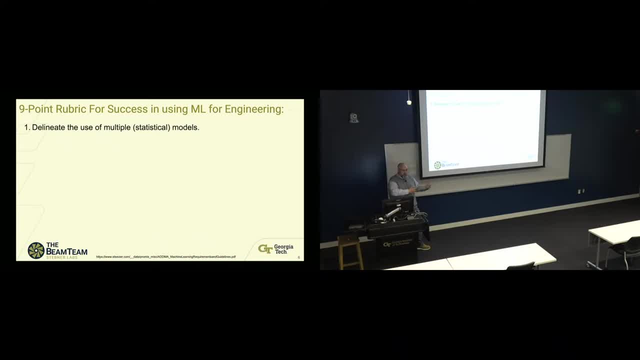 we have models for screening or making decisions about how to structure the main model that's going to be our predictive model that we use for the function, And then we may even have machine learning data analytics models that mine the model after it's been made right. 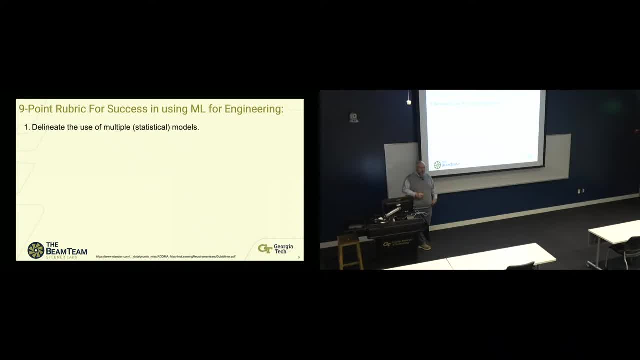 So you can often have three, four, five different models, Or we might have one model we want in the end, but we're going to make five different machine learning models and see which one works the best right, or something like that, And so we need to understand why we're making. 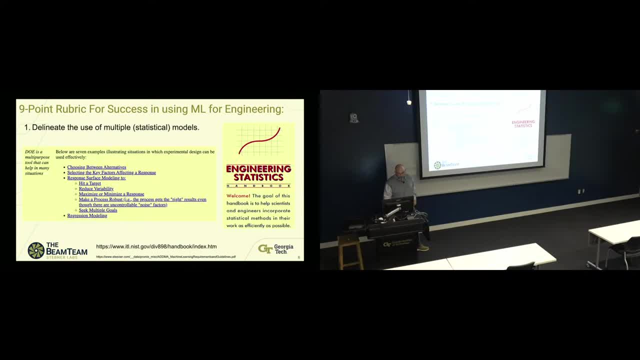 the model and how many models we're going to use, What models we need, et cetera. Really, I mentioned machine learning- is just statistical modeling in high dimensions. So in my class and in the journal and really with all my graduate students, we go back to the NIST engineering statistics handbook, which is 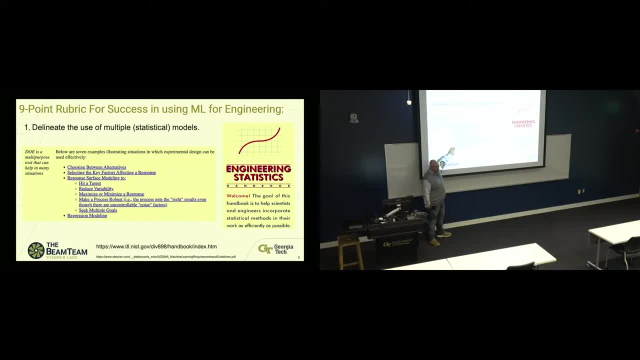 free published online. The reason you would use a statistical model really hasn't changed in 80 years, right? We can just do it in a lot higher dimensions now with machine learning, So we might need to choose between alternatives. select the key factors. 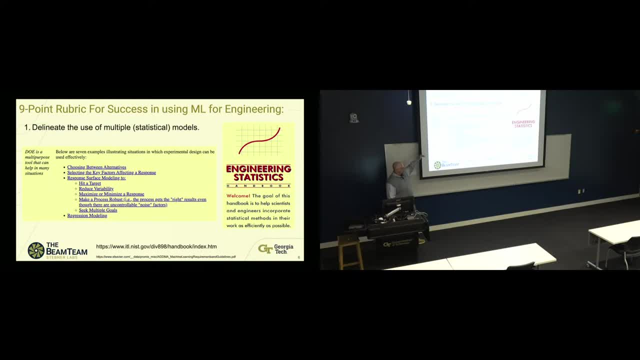 Hit a target, reduce variance or uncertainty right. All these different reasons we might want to make a model haven't really changed and we can really have a nice reference and list on the different questions we might want to ask and why we would want a statistical. 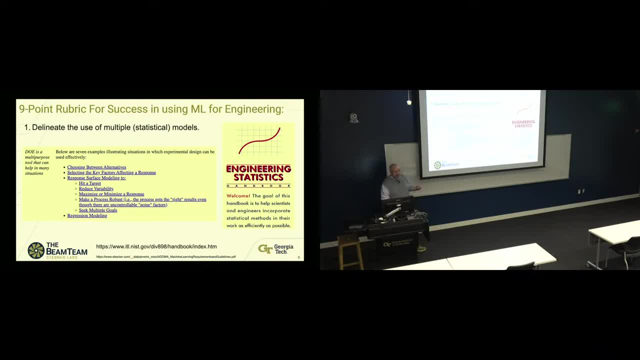 model. We need to think about that up front. We need to know the question we're asking and the answer that we're seeking before we just decide that we should machine learn it. The second thing, then, is we have to define the model, So machine learning cannot define. 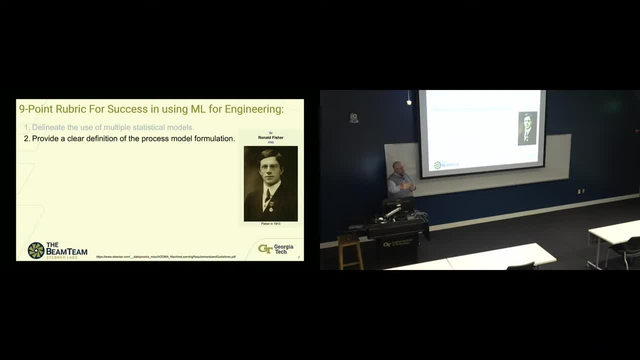 for the most part there are some advanced algorithms. There's really a frontier. where the computer scientists are is algorithms that can figure out what should be your inputs and what should be your outputs. But today, in practice, even in R&D in a university, most of us graduate students. 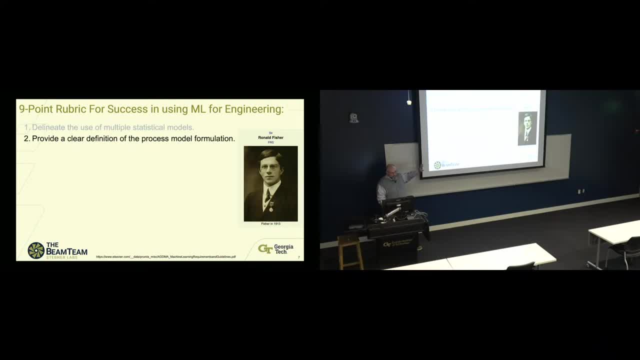 or postdocs or faculty need to provide for the computer before we construct the machine learning model. What is the process model, That is, what are the factors that we're going to vary in control? What is the response that we're seeking or want to optimize on? And then what are all the other things that are going to introduce? 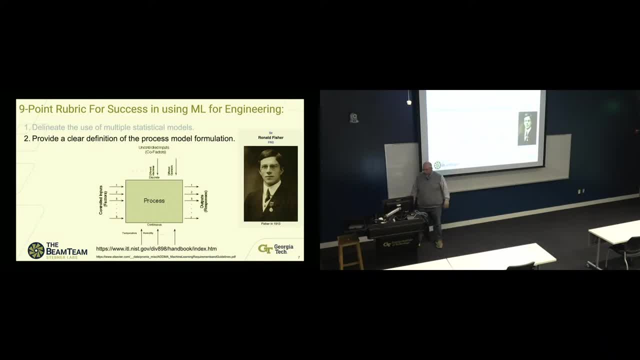 noise to my model that I'm not going to control but factor in to my data. And this is classical experimental design right, Your foundation of where you start with any experimental design, And it's no different for machine learning. If we don't know this picture, and sometimes 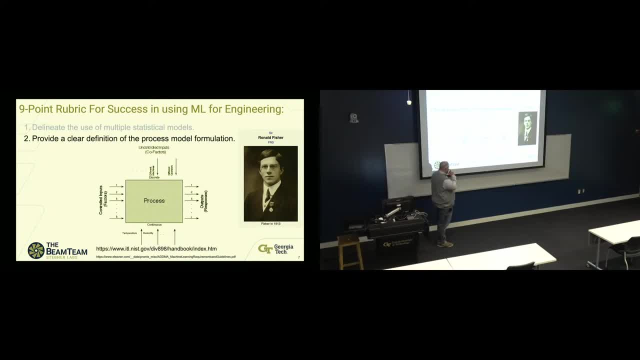 we use what's called unlabeled or unsupervised machine learning, and there everything's just a factor right, The outputs of the factors too, And so, yeah, I think that's a really important thing. So it's not different because there's these unsupervised, We still have. 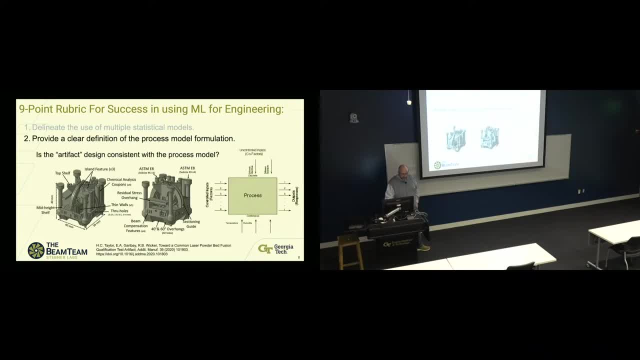 to know what we're controlling and what we're not controlling. Then we have to think about: are the experiments that we're doing, and in an experimental design? an experiment is not always something in the lab. That could be your DFT calculation, your 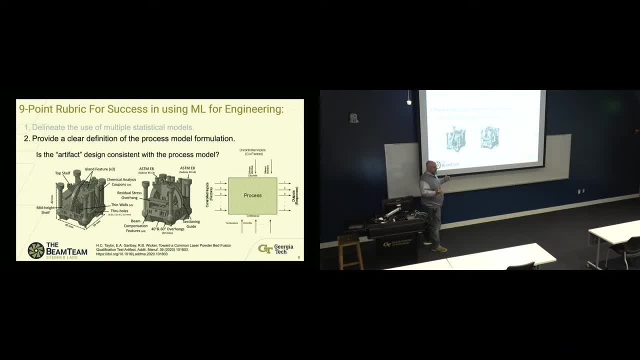 finite element simulation right. Anything that's going to be a source of data, is it consistent with the process model? This is an example I can pick on Professor Wicker at El Paso. he's editor-in-chief of the journal where I've been deputy editor. 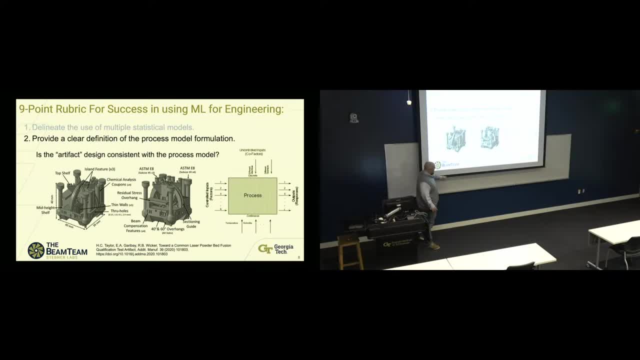 where we've developed a lot of this rubric And he has amazing expertise And they put out actually the companies here in Augusta, now that they've started up, And they came up with this artifact for metal 3D printing that they said if everybody in the world 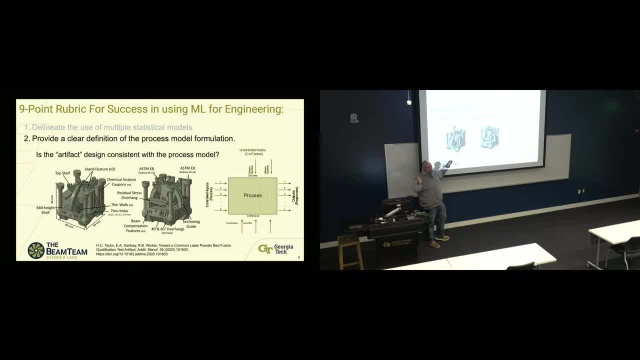 made this with every build they made and sent it in to us. we would build the database and we would be able to universally qualify and state the quality of any metal 3D printing. What they didn't think about is the fact that in this one artifact where we have tensile, 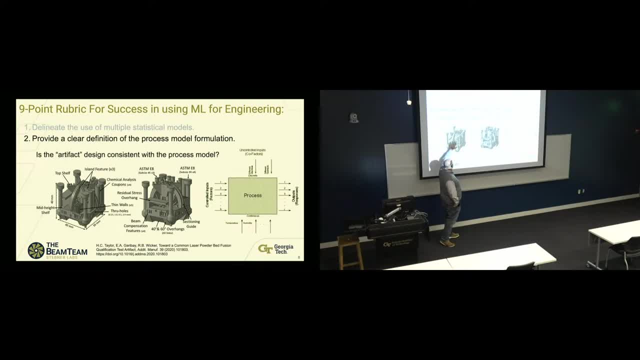 bars, fatigue samples, overhangs, overbuild, underhang, all these different features, microstructure. there's actually about 80 statistical models in this one artifact, all convoluted with each other, right, And so there's 80 of those process models in that one thing. And now 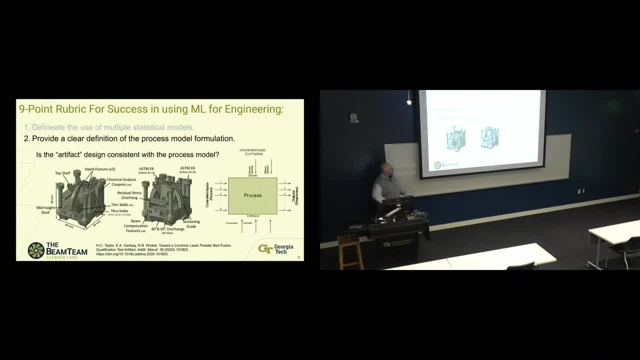 they're all coupled together, And so we've got to really put some thought into where we are in our development process and what we're trying to accomplish. Sometimes the right answer is we just need to, in 3D printing, put one track of material down and look at. 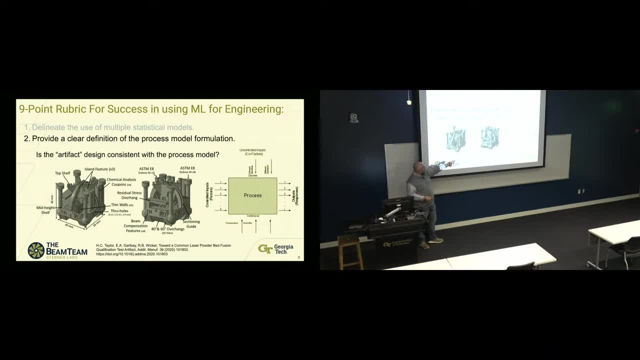 that if we're really early in the process so that we have fewer inputs and one output, maybe right Versus where we get to an actual fatigue performance, then maybe we need something more comprehensive. But this is really expensive. Each one of these artifacts takes their lab. 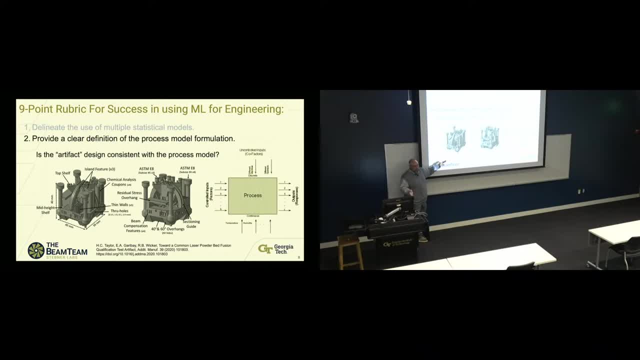 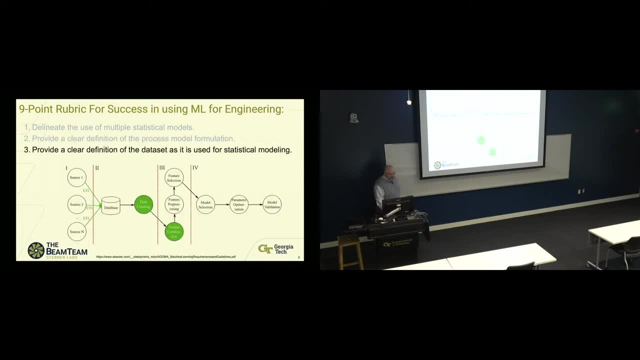 about two and a half months to fully analyze, And they have it set up with a lot of, you know, automation and highly trained workers, right, And so we've got to weigh all those things out in our process. Then we have to think about how we're going to define the 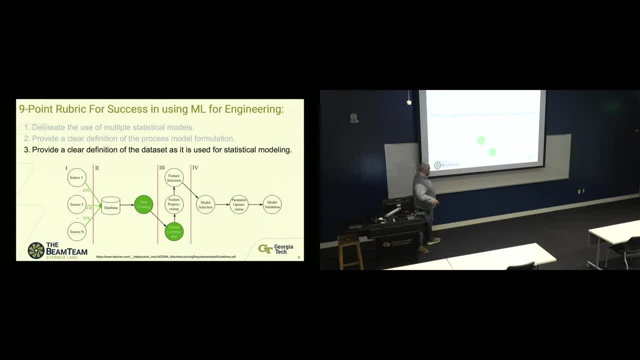 data set as it's used for statistical modeling or machine learning, And so this refers to the fact that you know when I run my DFT calculation, or I run my 3D printer, or I run my melting furnace or whatever you know CVD furnace, whatever it is I'm doing to make. 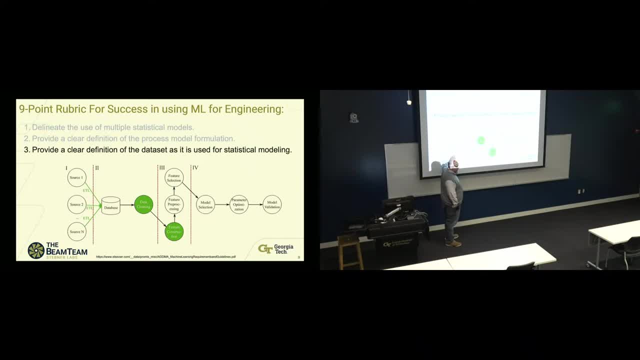 my material or my sample. a lot of times, the way that data is stored or logged by the computer that's running the instrument or the simulation is not the same as the way I need my data to go into my machine learning model. And this is actually, you know, still today in my lab. 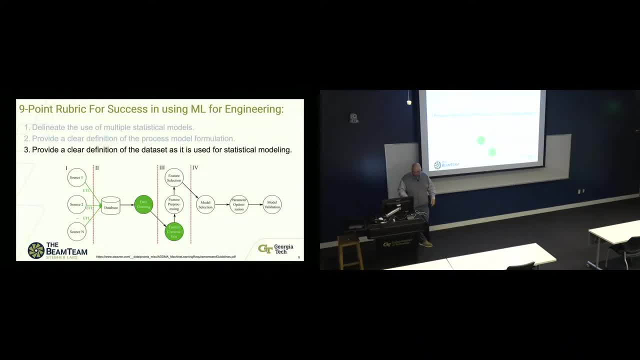 at least if a student is going to do we lost- oh there it's back. All right, A thesis and use machine learning modeling. they will spend about two years in these first three stages. Um, Let's see if I can breathe on it, as as we keep losing the video. 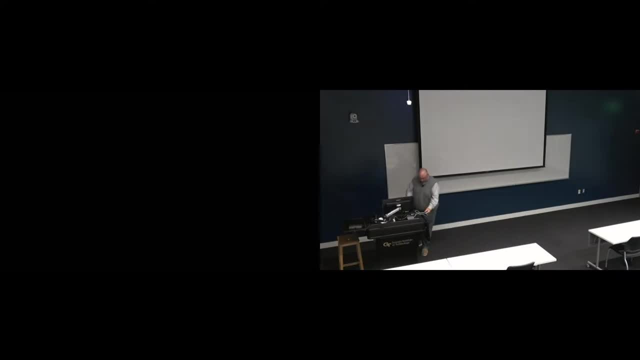 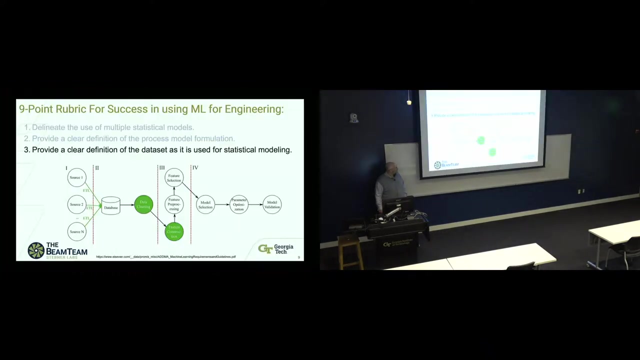 Let's see if it pops back again. Let's see if I can breathe on it, just right here. All right, We'll try unplugging and replug in here. There we go And then this creation and and interpretation in the machine learning model. they can often do in like 15 minutes. 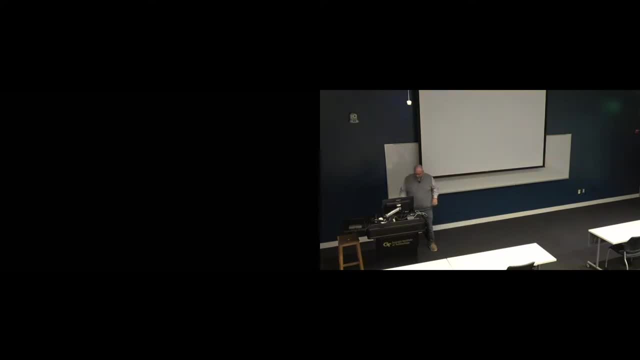 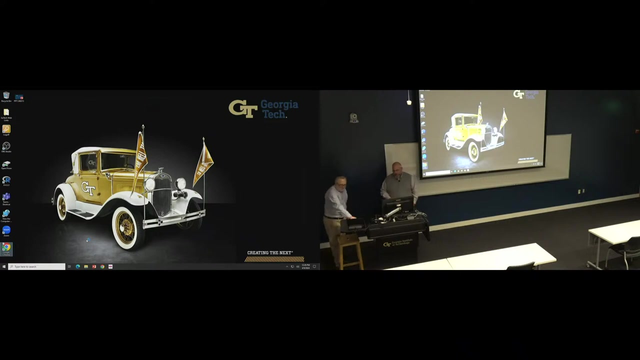 15 hours, right, All right. man, it's unusual to cooperate for like 15 minutes and then be fussy, right, All right. Okay, I wanna see if we switch back and try to keep going while we get that backup plan going. 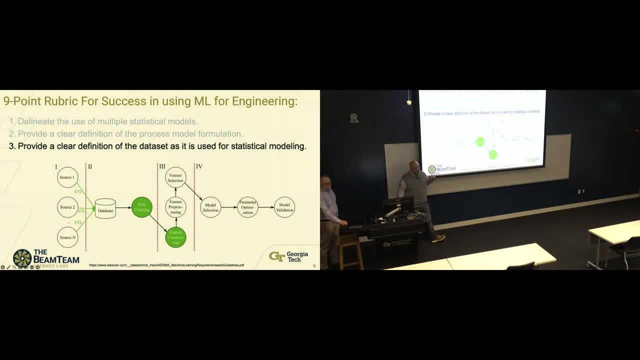 Okay, so the green are the opportunities for engineers and scientists to insert physics or base models or physics domain knowledge into this whole pipeline of getting from data you're collecting or generating to machine learning, modeling, right, And so this is where engineers and scientists really have an ability to innovate. 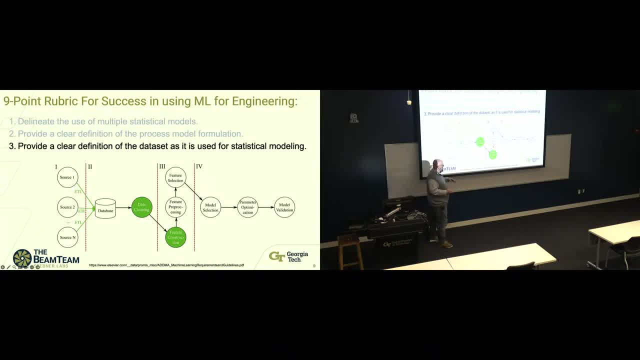 where no offense to any computer scientists in the room, but computer scientists, unless they've been trained in the domain, often can't make the innovations or don't think about innovations, And so a lot of what my group works on today is: how do we come up with general algorithms? 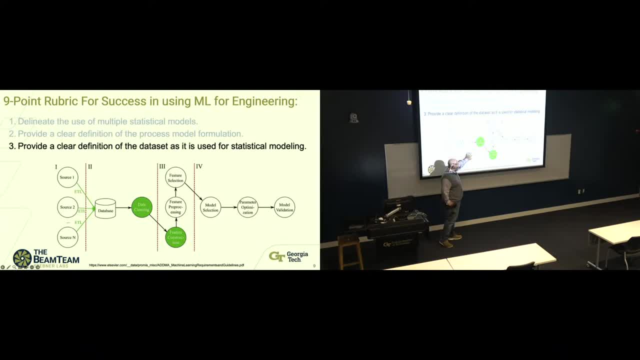 and constructs that can move data from one to two or two to three, so that this isn't always a manual ad hoc bespoke- I did it one time for this one data set process- but rather we can start to have AI techniques and elements that can help us here. 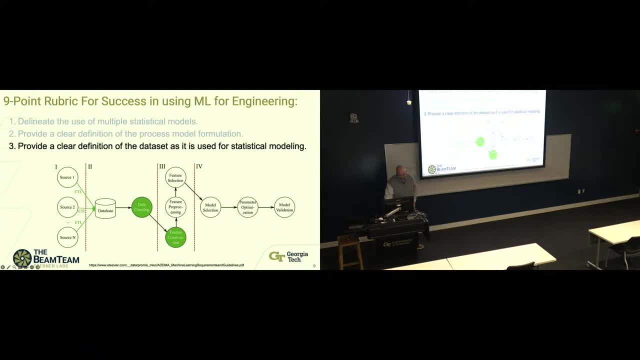 and then be connected to the machine learning modeling, And so that's, I think, another area. But from the rubric standpoint we need to understand how are we gonna get from the data, from the sources, to the feature selection? How are we gonna get from the feature selection? 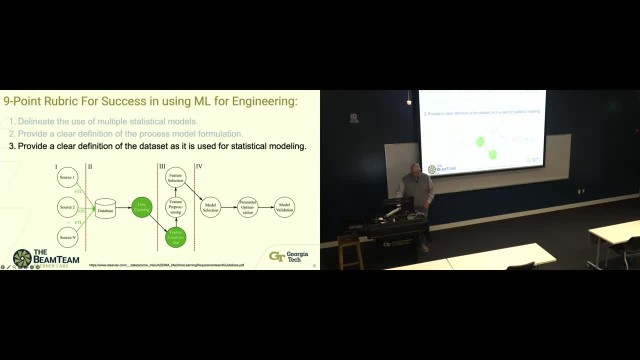 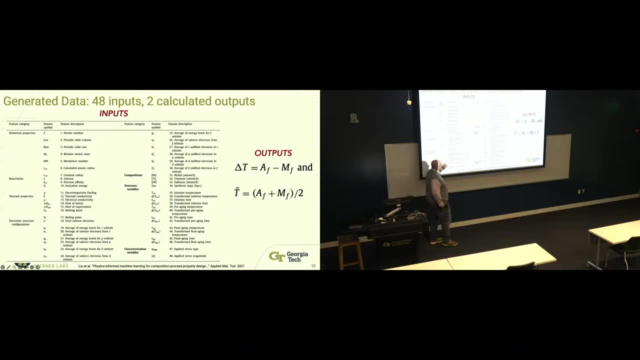 that's then used for the model in the machine learning part. And so one example there. I alluded to this earlier, but this is an alloy development program that we did. We have a publication on this. We were doing alloys made with combinations. 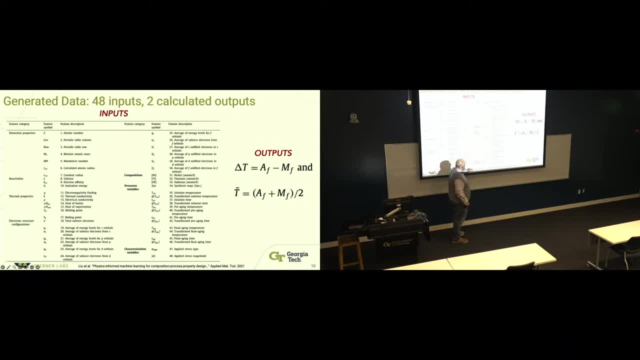 of nickel, titanium and hafnium. so just three elements. These are all of the process variables. so heat treatment times, temperatures, melting temperatures, melting times, And we only had two responses that we cared about. but then these are all additional inputs. 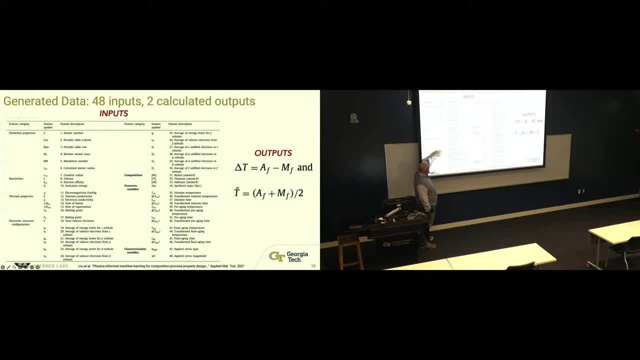 that we had based on the elements and how we were putting them together: electronegativity, thermal conductivity, electroconductivity. So for this one three-element problem of material design, we actually ended up with 54 possible features, including the inputs and outputs. 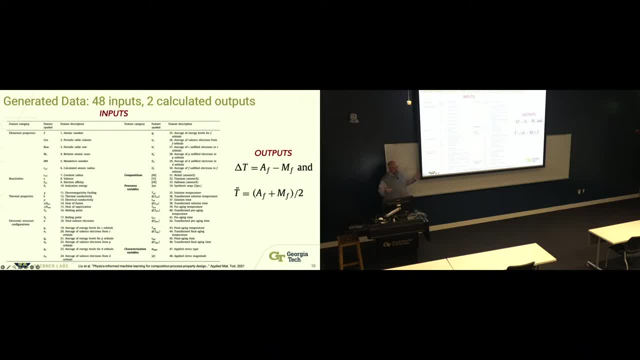 And so the amount of data we would have needed for a machine learning model for all of those is very high. We were typically needing like two orders of magnitude greater at least number of data points, And we only had a couple hundred data. 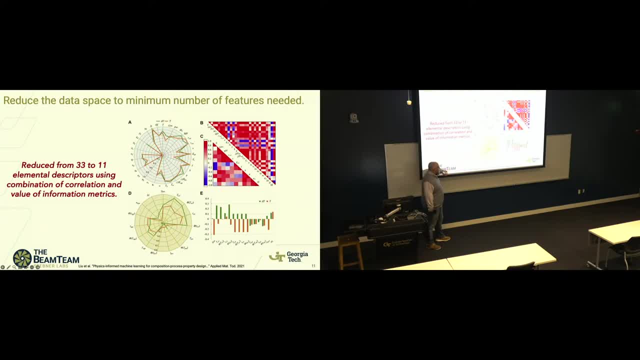 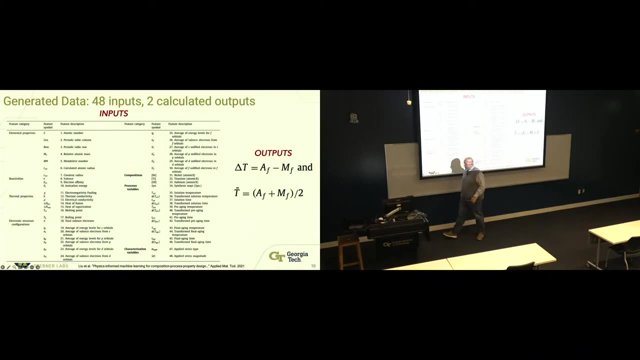 So the first thing we did was we built machine learning models to down select which features were most important to the question we were asking, which, in this particular case, was how to optimize these two temperatures of phase transformations in the material, And so we actually needed two different. 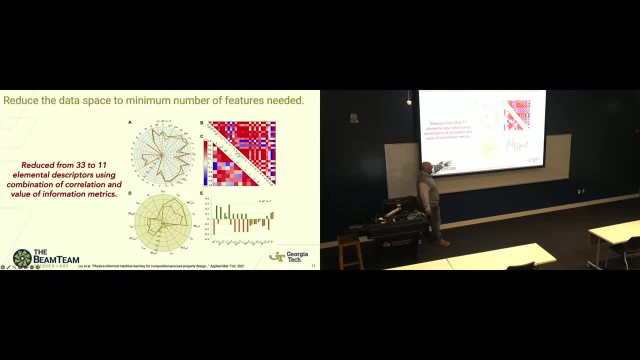 statistical models. We didn't even need machine learning for this particular problem. We used Pearson correlation and then a second maximum likelihood model, but we needed two different ones because of those features. the ones that dealt with the elements were what we call fully dense. 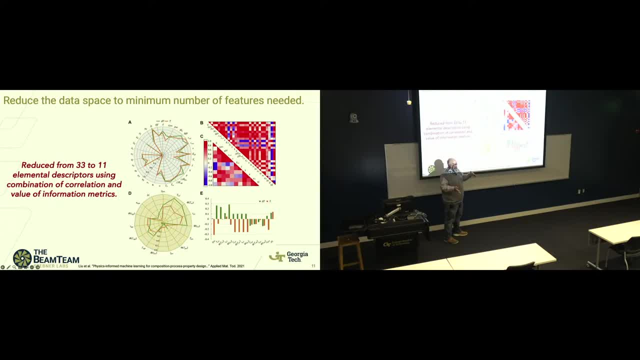 That is, we had an entry for every single data point, but the ones with the processing were not. We didn't heat treat every single material that we made with four heat treatment steps. Some of them only got melted, Some of them had one, some of them had two. 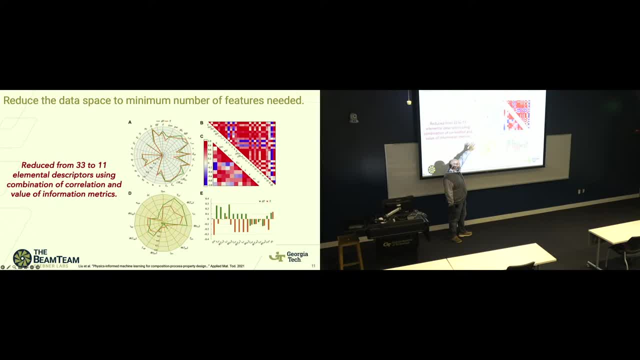 So we actually needed different. we need to understand one tool can't do it all a lot of the times. in statistical modeling, Some are really good at dense data sets, Some are made for sparse data sets and they have normalization or regularization built in. 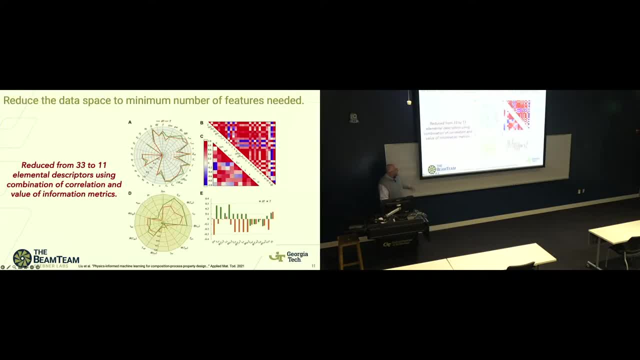 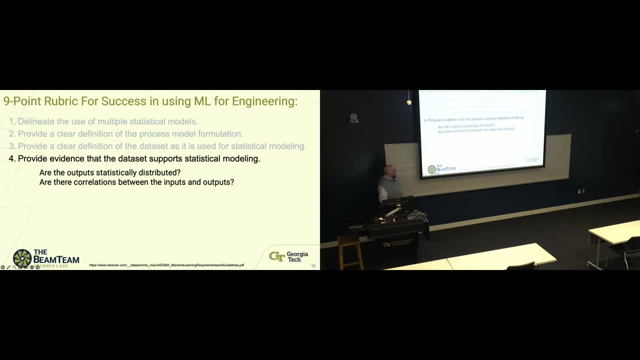 And so in this case, we were able to reduce, for the top, from 33 to 11 on the elemental, and on the process data, we were able to go from like 12 down to four or something like that. So then we need to ask the question. 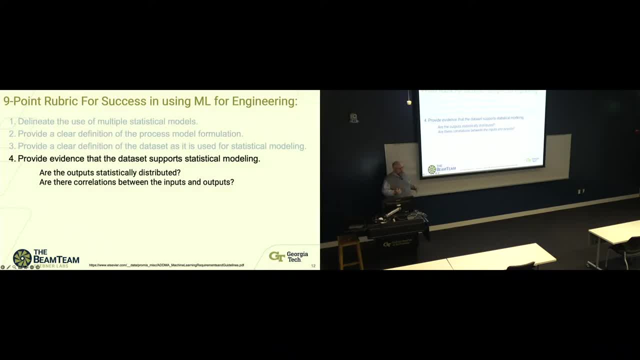 are the data good for statistical modeling, And so the main requirements here of statistical modeling- and they apply to machine learning as well- is that the outputs, or the things that you want to measure or answer questions with, have to be statistically distributed If they're discrete or outliers. 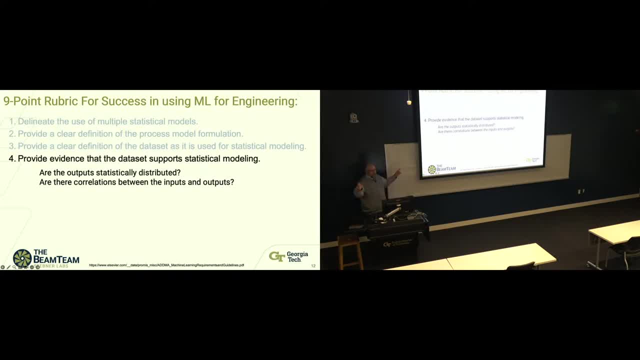 your model of statistical distributions is not gonna find your model of statistical distributions is not gonna find your model of statistical distributions is not gonna find those points, or it's gonna ignore those points or possibly be heavily biased away from those points. And then there also have to be correlations. 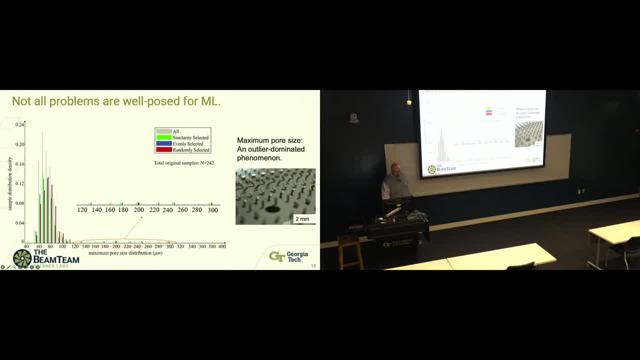 between the inputs and the outputs, And so this is an example picking on myself now. When we started the Center for Metal 3D Printing to help companies in the aerospace industry in Colorado, one of our ideas we took from the composites industry, which was: could we come up with a data? 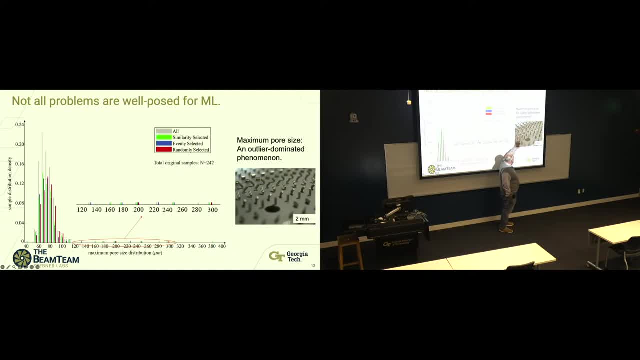 some kind of benchmark set and in this case we printed 600 of these pins on different plates and we printed some plates exactly the same way, others with different variations, And we wanted to find like the 10% of the data that represented kind of the mean and the tails. 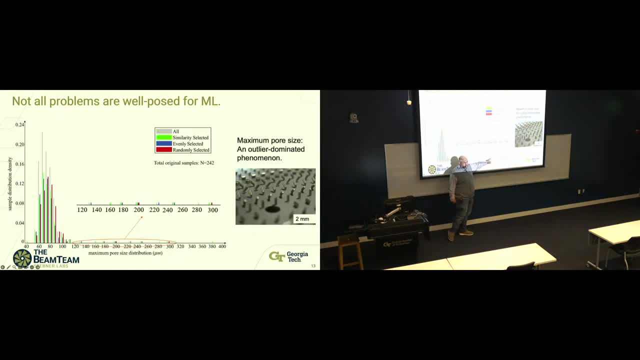 and the ones the company doesn't wanna make. are these outliers up here on the big side. These are big defects that they don't wanna be able to make. And can we pick out of the 600 parts 15 parts that they could print before every service call? 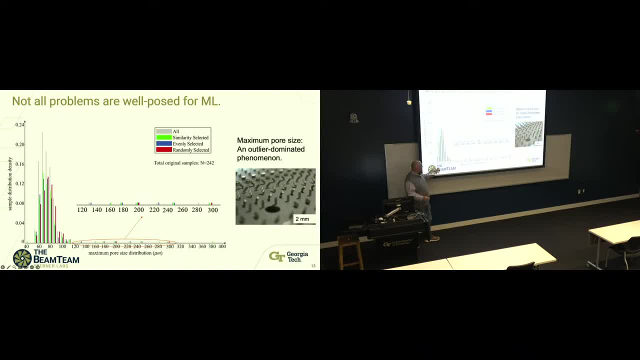 after every service call, after every service call, after every software update, and if they check out and they say parts two through 12 fall in the mean, part 16 gets this result. part one gets this result. they know they're okay. 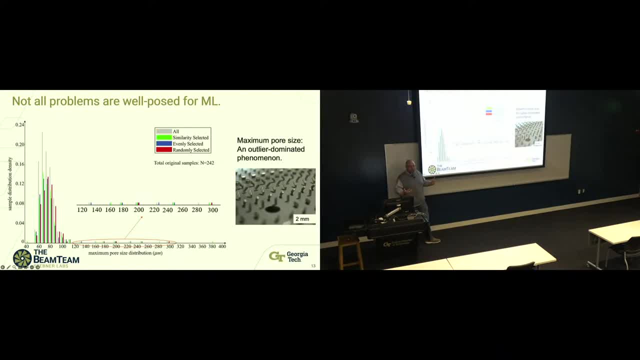 They know the quality of their process hasn't changed and they can go on believing that they're qualified. The problem is the machine learning to this response on porosity in the parts wants to model this distribution. This is the statistical distribution. It doesn't wanna model this outlier. 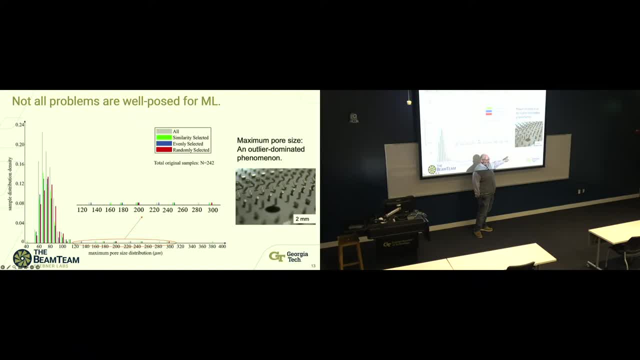 which is the worst case for the company and the one they need to know they can avoid and not make and deliver to Lockheed Martin or whoever they were making the part for. And so the initial attempt to build this machine learning quality model failed. But then we decided, and so machine learning. 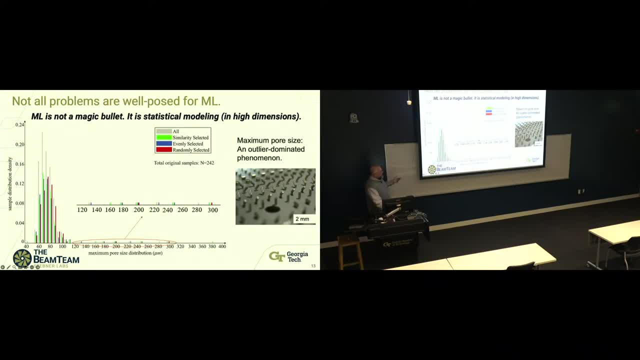 can't just learn it. for us, and often the way we ask the question also matters, And so I don't have the second slide here. but we ended up solving the problem by saying, instead of trying to build a model that'll tell me, 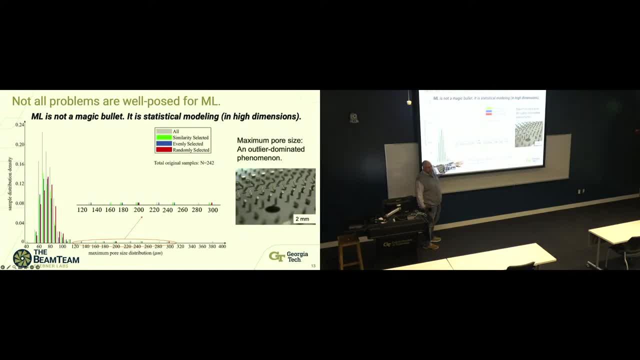 what the pore size is, given the parts, the orientation, how it was made. can I just build a model that says fail or pass and build my model to that? And now, by making this categorical, it could predict will it be within the distribution? 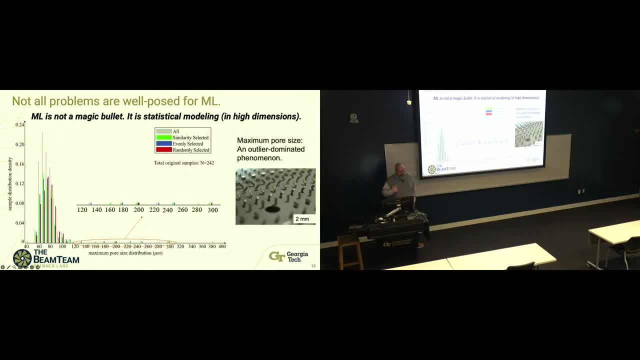 or will it be an outlier? basically is what we asked the model to do And now we can have a quality model that works for the company right, And we actually made it: red light, yellow light, green light. We had zero to 100 was green. 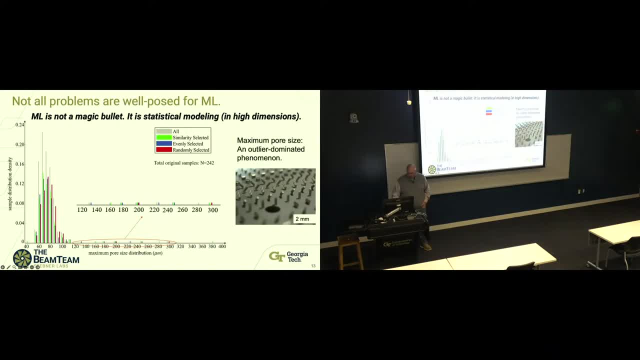 100 to 200 was yellow and we had a red light, And that's something the technician could also want, And that's something the technician could also want, And that's something the technician could also want. Okay then we want to know. 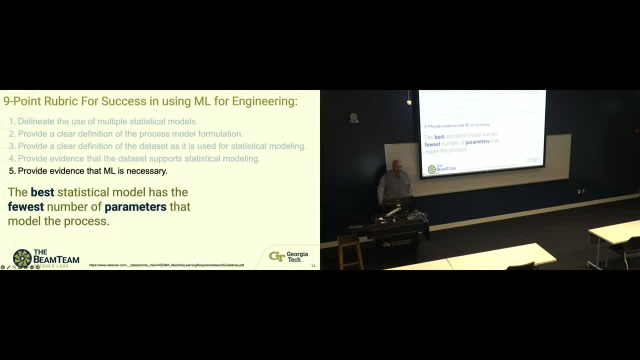 that machine learning is necessary. And this goes back to a foundation in statistical modeling. which is the best statistical model has the fewest number of parameters that adequately model the process or answer the question you're trying to ask, And so this one actually came out of. 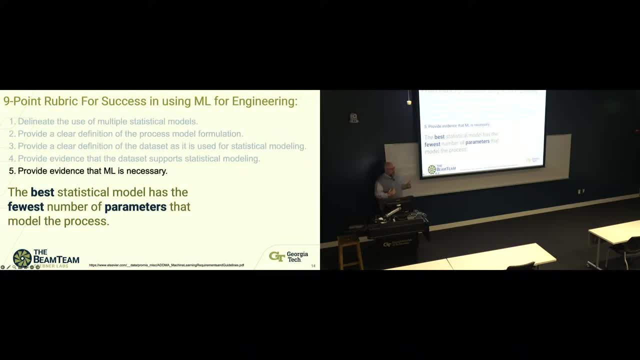 the editor for the journal role where- 2012 to 2017, we were getting a lot of submissions of people saying I used the latest machine learning model published by this computer science group. therefore, this paper should be published right And at the time. 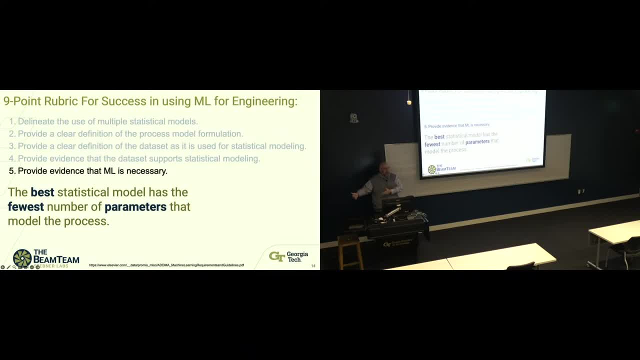 engineering community didn't really. that sounded like reasonable, right? They're using the latest advancement in machine learning on this problem. they showed that it worked. that seemed pretty cool. The problem is we started realizing people were using neural networks with 40,000 degrees of freedom. 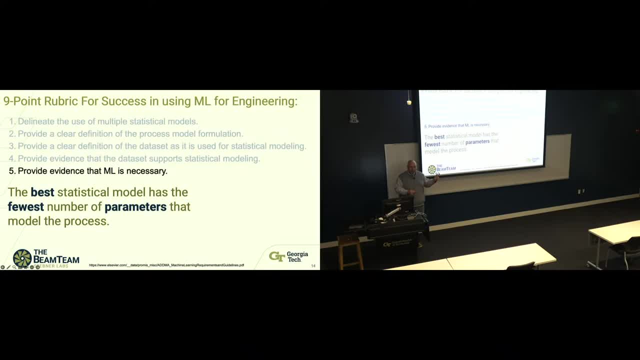 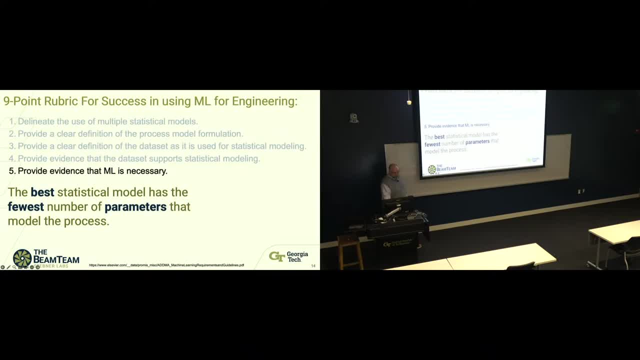 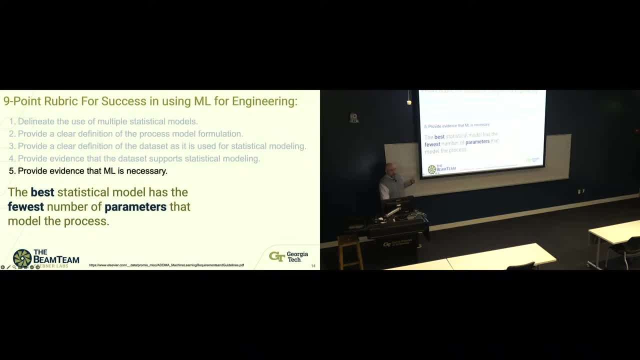 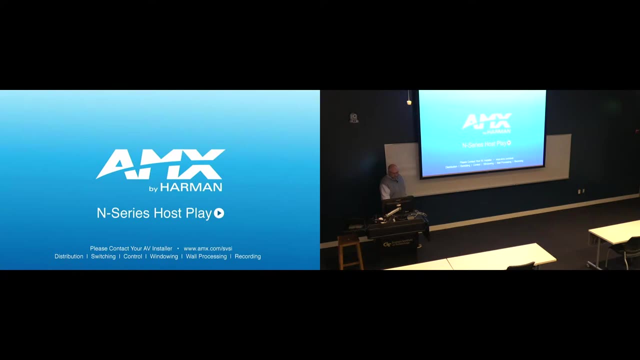 and realize. the simplest model, at least for the purpose of answering an engineering science question, is the one with the fewest number of parameters, And that just goes back to this bias, variance trade off and having a well optimized model picture. All right, we got that far. 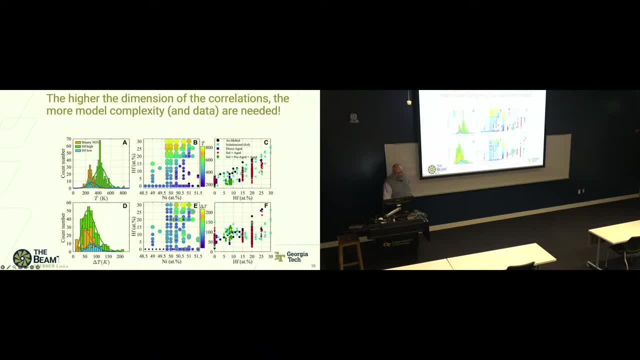 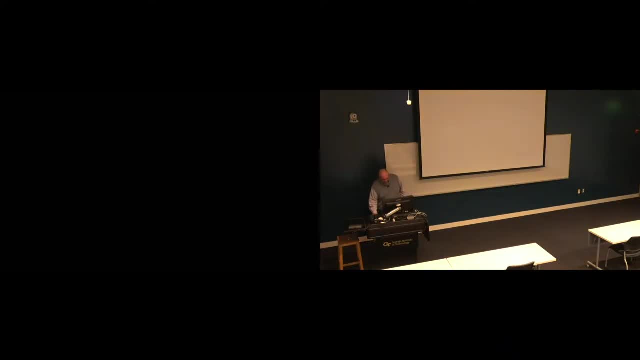 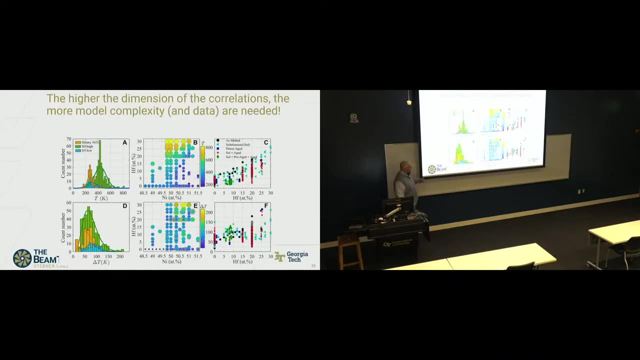 Let's see. Oh, pop back, Okay, Okay. And so how do we examine whether or not this is necessary? Let's see if we can get back here. It seems to work with technology, Right, All right, Okay. So how do we answer this question? 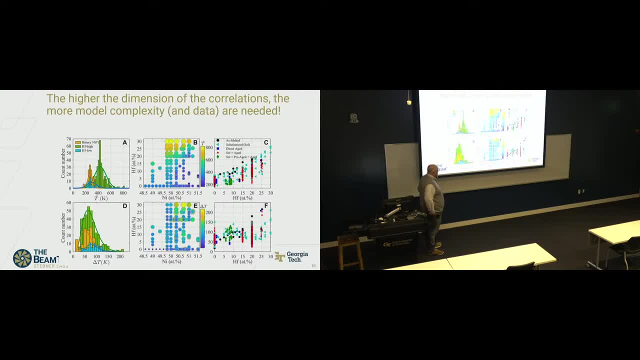 Is machine learning really necessary? And the easiest way I've found in it, at least the way we use in the class. there's lots of techniques being developed to answer this question. The simplest one is to start with lower dimensional plots and and okay. 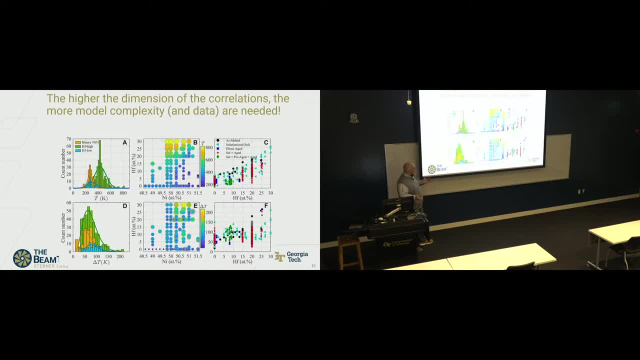 visualizations and say: do they adequately and fully describe the trends in my data or not? And so we can just use two-dimensional plots, like plotting X versus Y, and here we can see there are trends, but these vertical lines show that something. 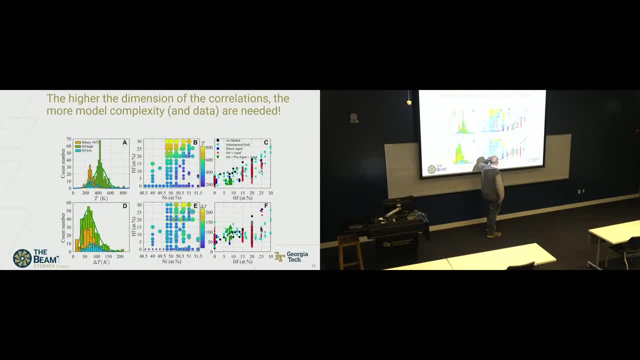 is completely not modeled by that two-dimensional model, Or we can go out into four-dimensional models. So here we have X, Y, marker, size and color. We have four dimensions and again we can see generally there are trends, but there's some yellow dots hiding under here. 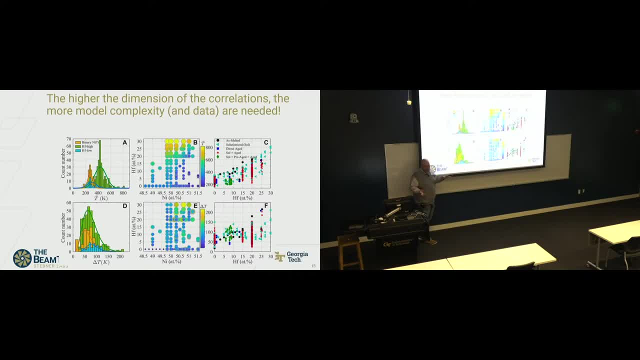 some blue ones up here. Those four dimensions aren't enough And if we can start to get to five, six, seven dimensions or pairs of, we do pairs plots where we have maybe all 15 variables and we look at the two-dimensional relations of them all. 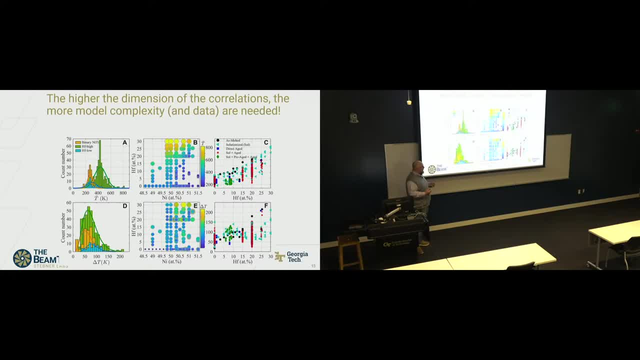 and we see that none of them are complete, then we can start to believe: okay, there are trends there and there are obviously models of the data that can be made, but I can't make them in two, three, five, six, seven dimensions. 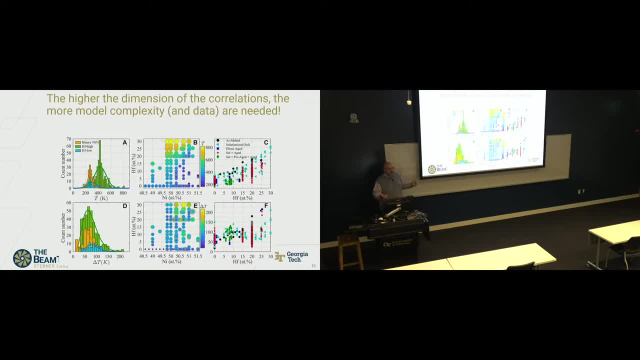 I need four or five dimensions. I need higher dimensions. That's a good indicator. I probably should try some machine learning techniques or some higher dimensional statistical modeling techniques. And then there's been other times where students go through this exercise and find a three-dimensional model works. 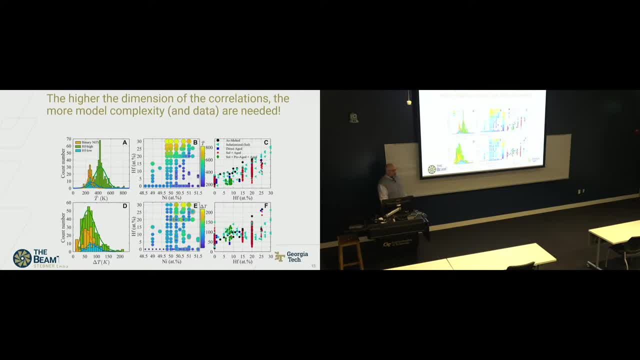 and we can run regression and away we go and we've got a simple model. It works and it works on few numbers of data and even though the student isn't happy that they didn't get to machine learn it and write a machine learning paper. 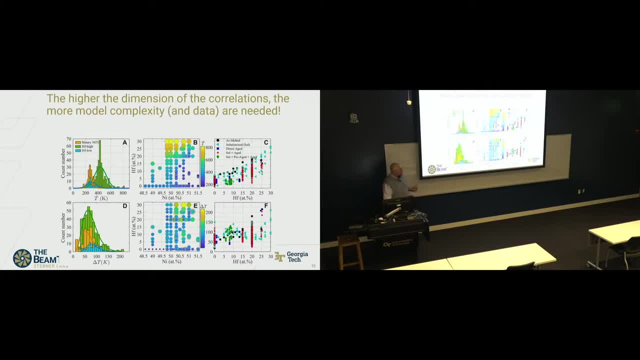 they actually solve the science or engineering question efficiently and effectively and they don't need thousands of experiments, which is also good. Another example of where we can use physics to help this process. I'm using the wrong computer, All right, let me close that one. 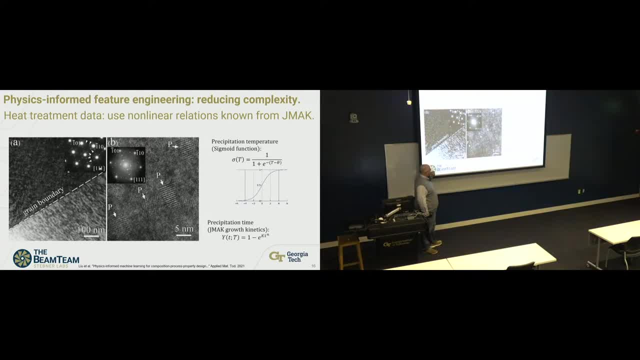 is that alloy development paper I was talking about, or project that I was talking about? Even after we down-selected to 13 features out of that one set, we still found that when we did that, we still found that when we did that we made the model. at first it wasn't working well. 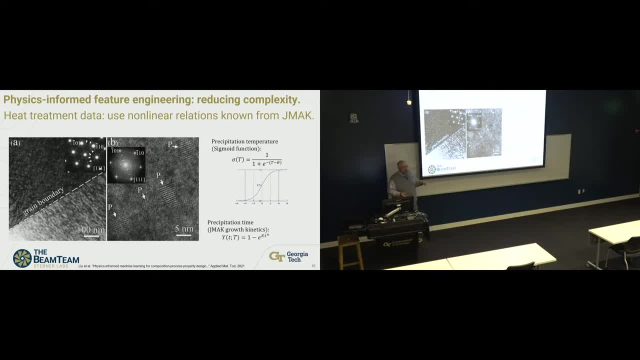 In that particular project we had 520 data points. It took us about 12 years, and I don't know how many millions of dollars, to generate those 500 data points right. Nickel, titanium, hafnium are not cheap elements. 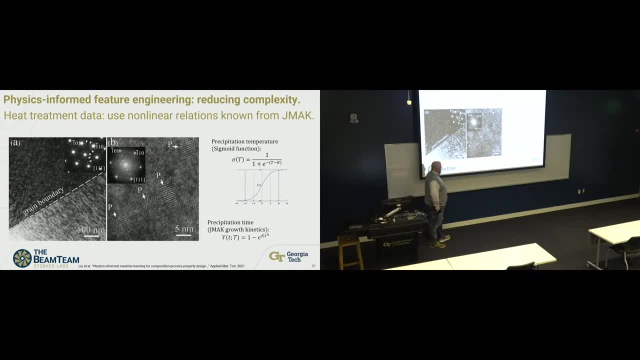 melting them, all the characterization, and so we didn't have another 10 years to add another 500 data points to help the machine learning work better. but what we figured out was those heat treatment data from melting the alloy, homogenizing the alloy. 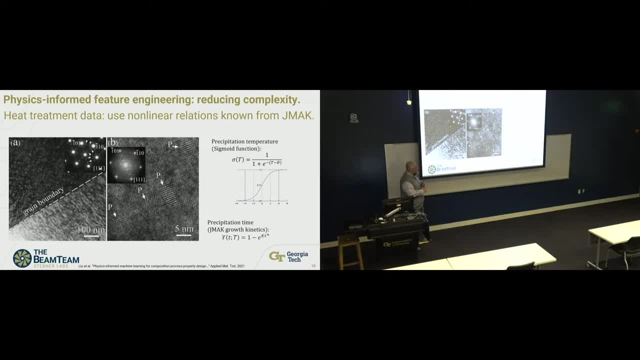 growing precipitates in the alloy right. different phase transformations. instead of using the data of the times and temperatures from the furnace controllers, there were actually 100-year-old, really well-known models in physics and chemistry that we could use. that knew the nonlinearities in the data. 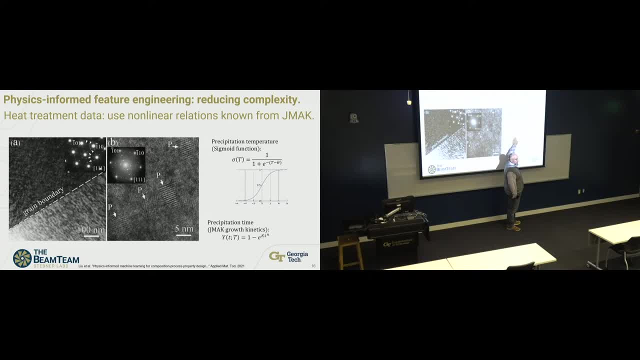 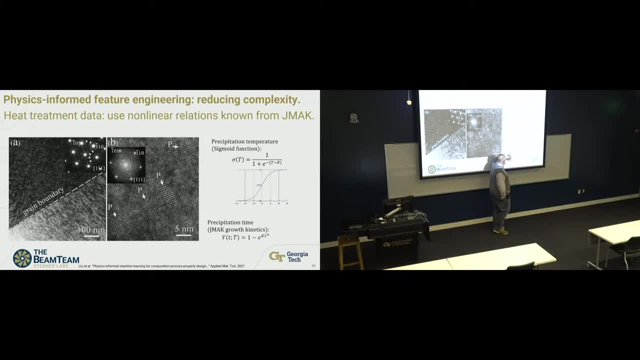 Gradually happens and then, above a certain temperature, it happens really fast, right, kinetics. And then, similarly, once it starts to happen, first it will happen fast and then it will decay in time, right? so JMAC growth kinetics. 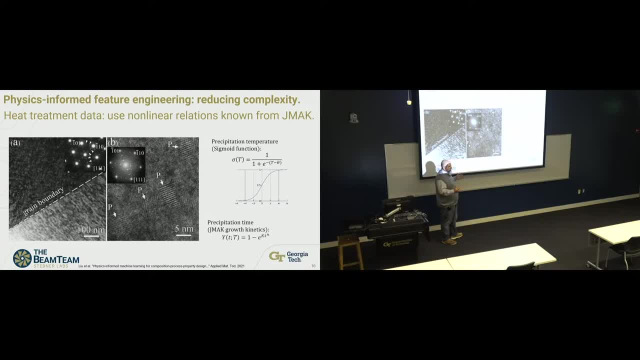 So if we now take the temperatures and times from the furnace controllers and take them through these nonlinear functions that we know from 100 years of physics, right, we can actually linearize and effect the data that the machine learning model works for and reduce the number of degrees of freedom. 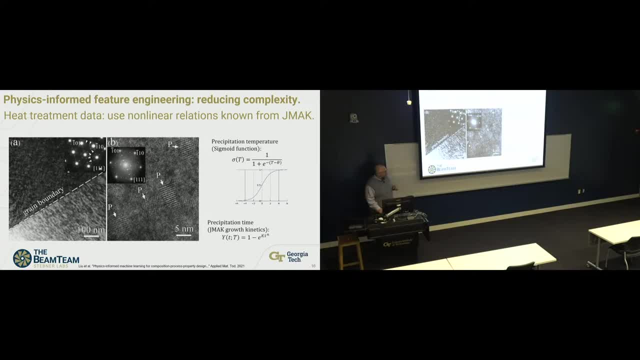 and the machine learning has to fit, And we'll see in a few more slides the final results of before we did this transformation and after it, and how we were able to use the same 500 data points and get the machine learning to work 100% better. 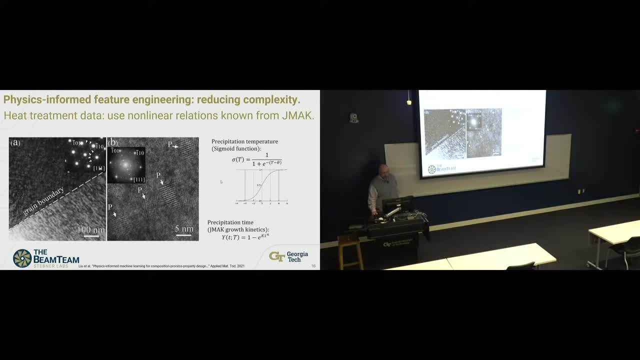 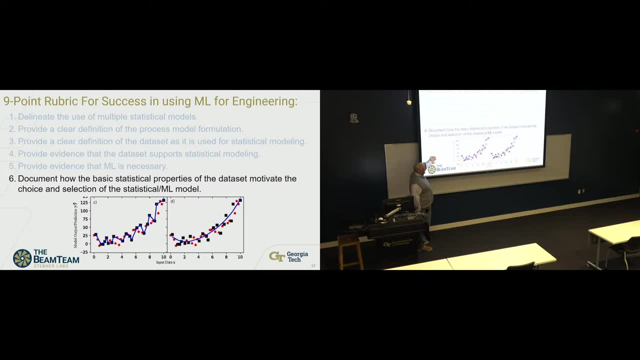 in one of the models, which is pretty cool, by inserting our physics knowledge into the data processing steps. All right, then we have to be able to select the right kind of machine learning model and the right numbers of degrees of freedom in the machine learning model for our data. 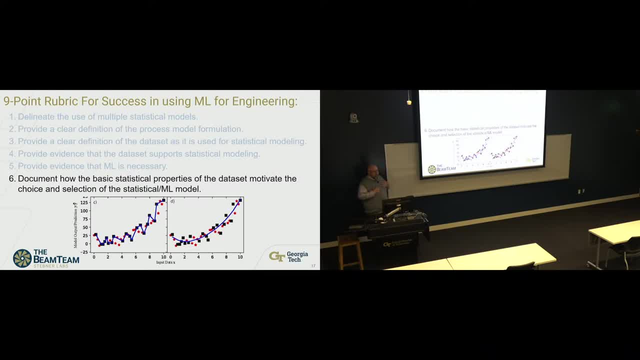 So we need to. as engineers, we don't need to understand how exactly the machine learning model or theory was derived, but we do need to understand that. if I pick up a neural network with five hidden layers and certain number of nodes in each layer, 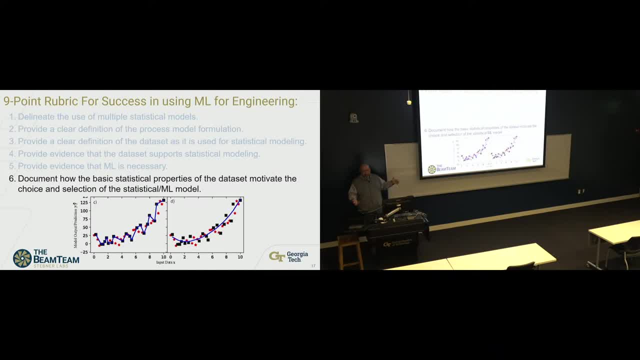 I'm gonna have ballpark 2000 degrees of freedom in my model. If I only have 20 data points, that's probably not a good choice for me, right? But if I'm gonna have, if I have 5,000 data points, right. 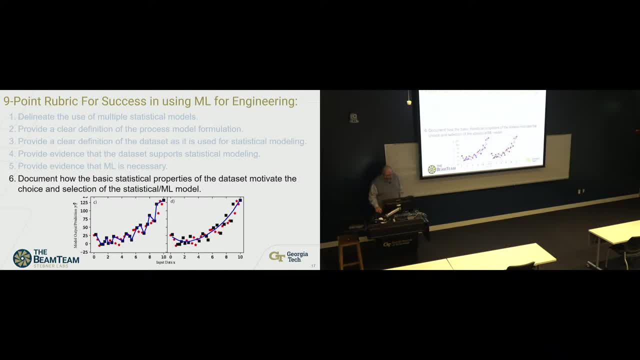 Okay, now I can start to think about that because, you know, maybe not everything's orthogonal and I don't really have that many dimensions right. So as engineers, we need to understand a basic sense of this picture, the different algorithms that are out there. 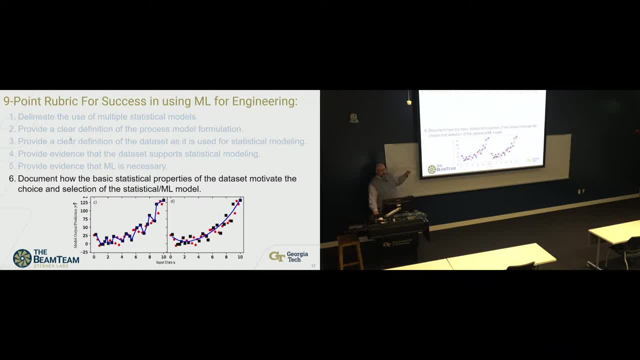 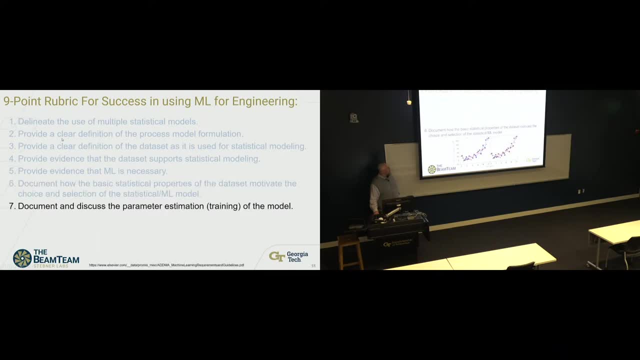 the number of degrees of freedom we introduce by making different choices in the hyperparameters, which are the parameters of the algorithm that the machine learning doesn't fit, or learn by training our data, and we need to understand how to apply those. All right, finally, for the journal and all. 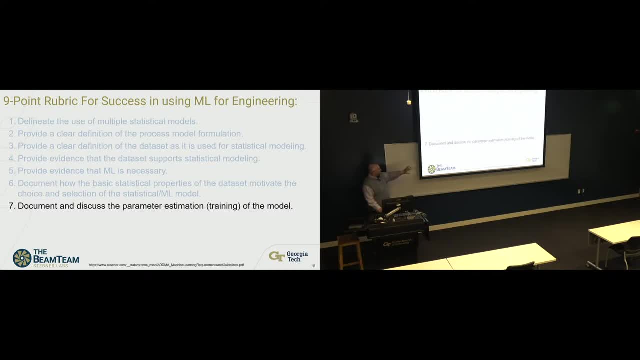 of our students. we require that we document how we train and estimate and choose parameters of the model. So what optimization scheme was used, You know? did we use a right? did we reserve some data to test? Always an important step. We believe it or not, still get a lot of publications. 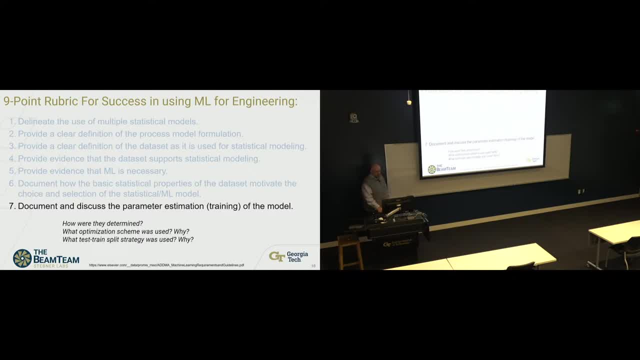 to the journal, where authors don't do that. They train on all their data and then show they can predict the data they just trained on, sometimes All right. And then, finally, we want to assess the model performances. So this is where verification, validation techniques. 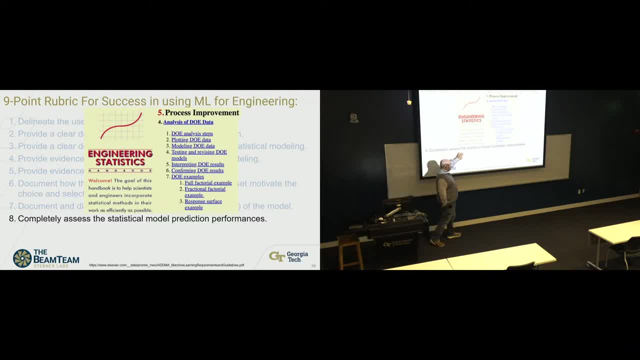 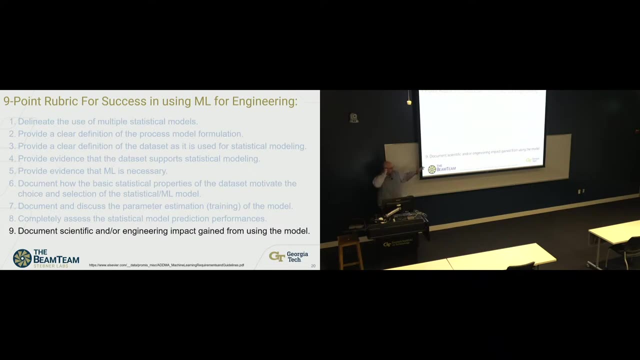 come in and again, the techniques really haven't changed from what we do with traditional design of experiments. We're just doing it in higher dimensions now, And so a lot of the same techniques of residuals analysis still apply. Finally, what we require for the journal now: 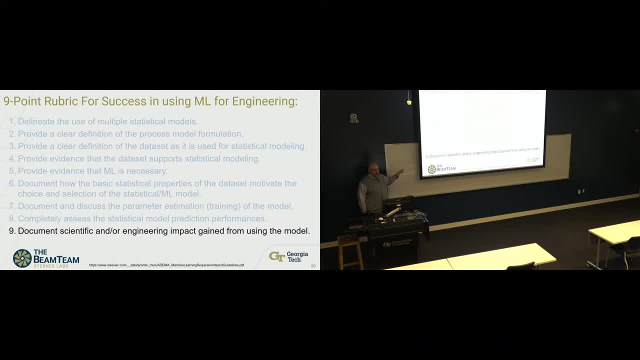 and I require of all my students, before we submit a journal publication from work we're doing in our lab, is: did the machine learning actually get us somewhere that we couldn't have gotten without it? right? and so there's. and not only that, but a second part of this. 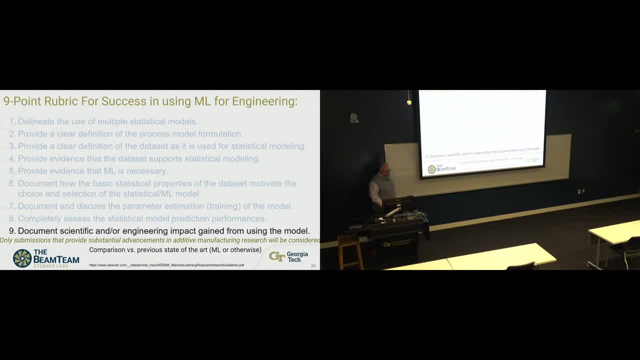 I don't know if I have it on here. yep is yep, so we can compare against previous state of the art. but also, where does the machine learning fail or where is it not meant to work? Documenting, that is almost more important. 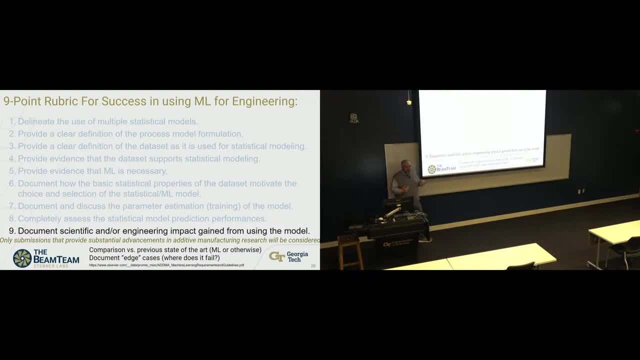 than documenting where it works, and this is counterintuitive to new graduate students. Nobody wants to say that the thing I did doesn't work somewhere, but actually it's the way you're gonna increase your citations and the impact of your work, because it gives others a clear picture. 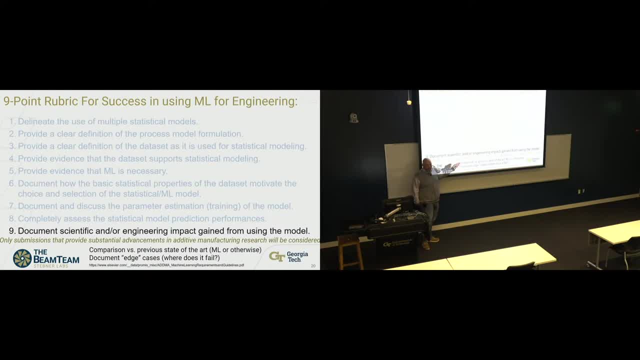 of what they could do next, to build upon your work and take it into a frontier where it hasn't been before. and it also helps us ensure as a community that somebody doesn't pick up your machine learning model thinking it should work for this. use it, apply it, build a bridge with it. 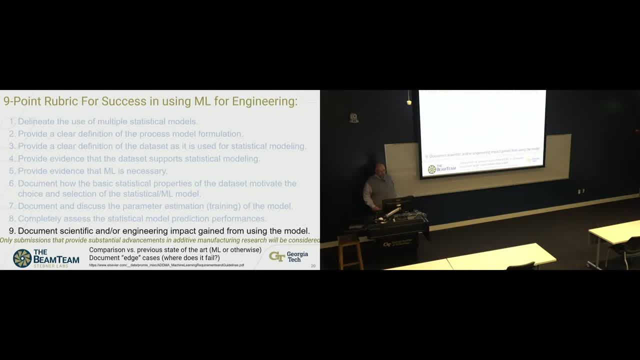 and then you know people driving across the bridge you know have problems a couple years later or something like that, right. so this is an important part of all. statistical modeling is documenting the statistical domain that the model was fit to right. 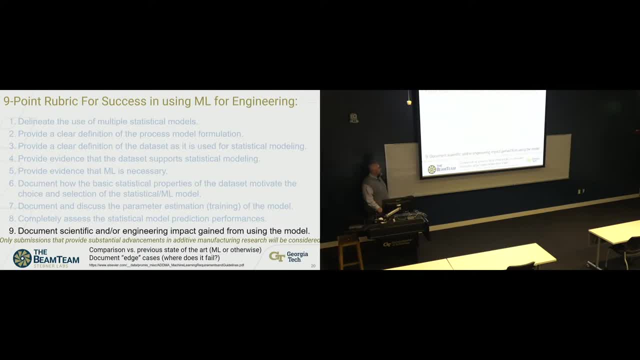 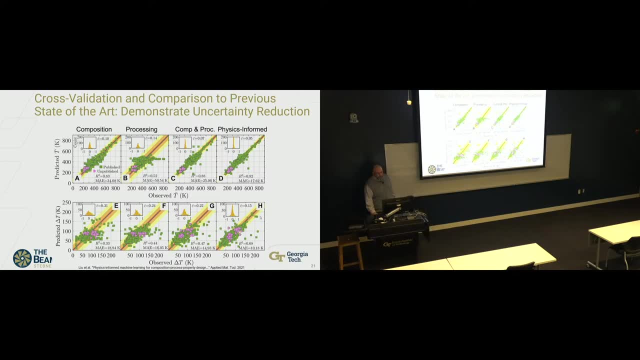 and that doesn't change just because we're machine learning it right. And so this is that example from that alloy design project that I was talking about, and so this column here is the model where we use all the composition and processing features, the down-selected ones. 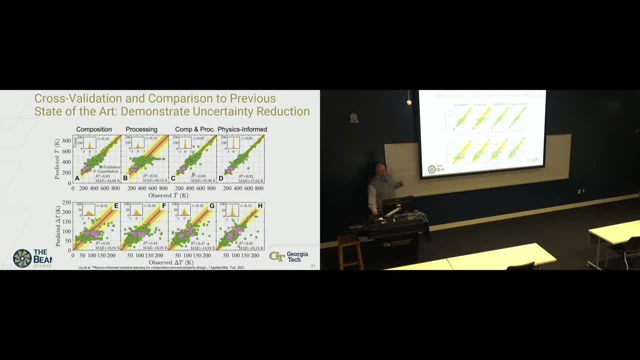 and for one of the temperatures it was working. so here, if it works, it follows this diagonal line where the predicted and observed, especially the testing data, and in this case the pink triangles, are actually blind data. they're data that we made afterwards. 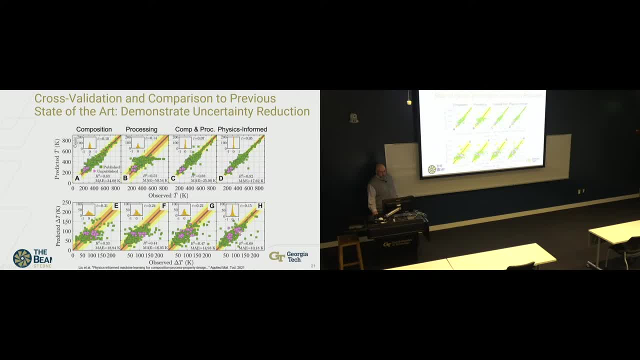 with the model predictions. but this second one, the range of temperatures over which the phase transformation happens, wasn't really working at all yet. but when we use those physics to pre-process the data that I showed, the JMAT growth kinetics, we now have both models working. 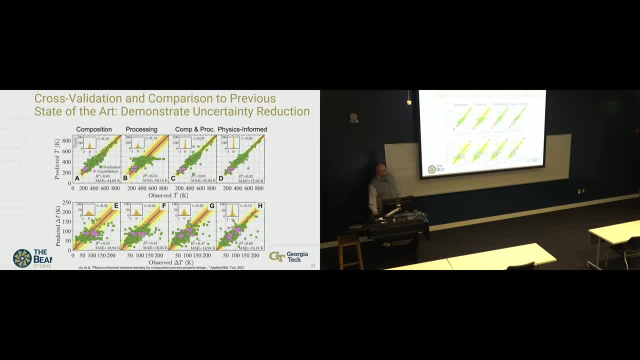 that we cared about both responses. This one got better and this one went from pretty much not working at all to working fairly reasonably well, and this has been something that in 70 years of physics-based modeling, we haven't been able to model yet to this well, so this was a good improvement. 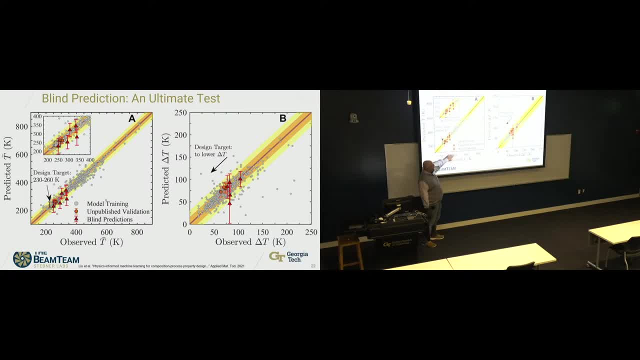 We then went and did what we call blind predictions. This is a great way, if you can afford it, to really demonstrate your engineering impact. Can I now take that machine learning model that I made and not just the test data that I've removed? 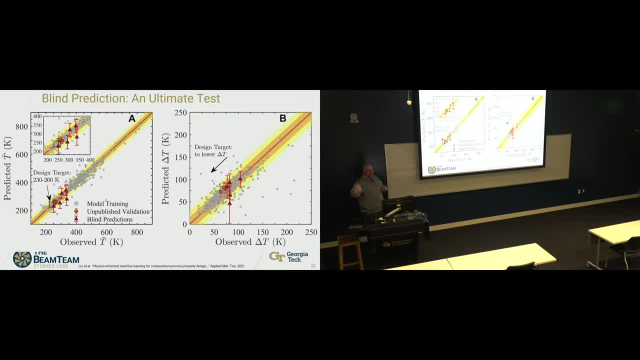 from all the data that I had available at the start. but can I predict new things that I haven't done yet? go out and do them and do they work. So that's what we were doing with the red triangles here And then, finally, where does it not work still? 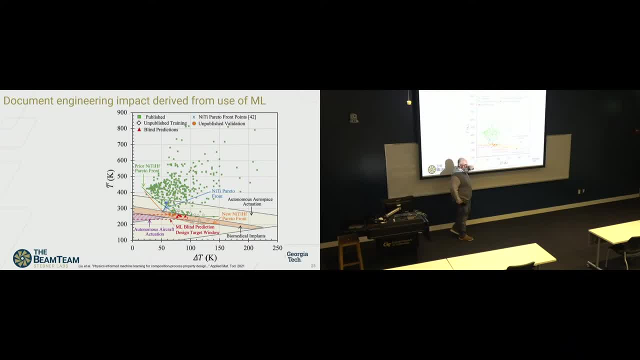 And so this is, in this particular case, the alloys we were developing. we were trying to get an alloy. one of the holy grails in shape memory alloys- which is a field that I work in aerospace- is if you can get an alloy where the phase transformations 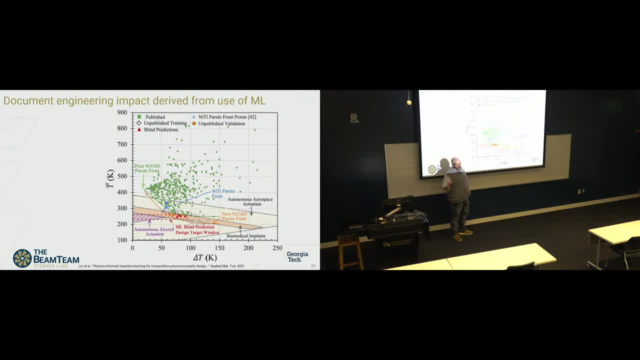 happen in this purple triangle. you could have a wing change shape between being on a tarmac and at altitude, without any electronic control system, Just the phase transformation in the material and the temperature change being zero Celsius or warmer on the tarmac and whatever it is minus 50 or lower. 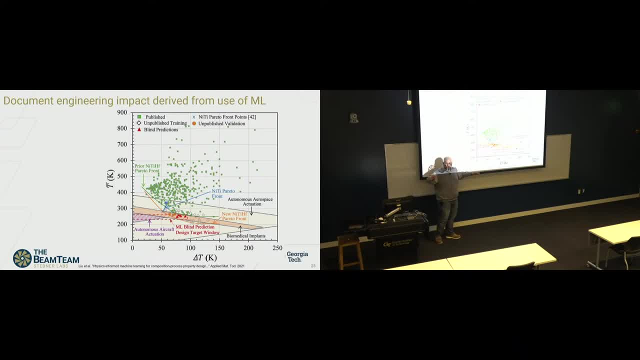 up at 30,000 feet in our atmosphere will allow your airplane to morph for flight versus takeoff and landing. We couldn't get there with this model and that was important to show because this is still something people can pursue, probably by going outside of nickel, titanium and hafnium. 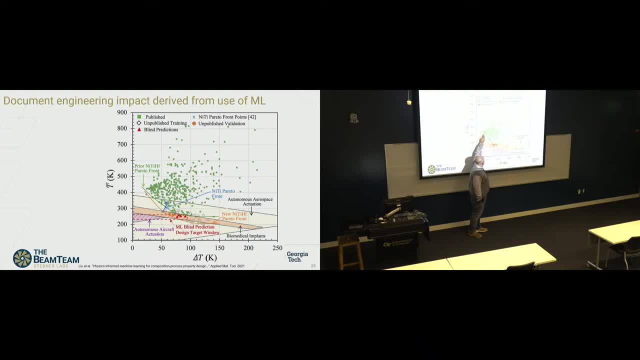 But we also showed where the previous state of the art of physics-based and machine learning was with the green line and how far we were able to move that line with our new approach of processing that heat treatment data using the JMAT growth kinetics. And it did get us into one new application. 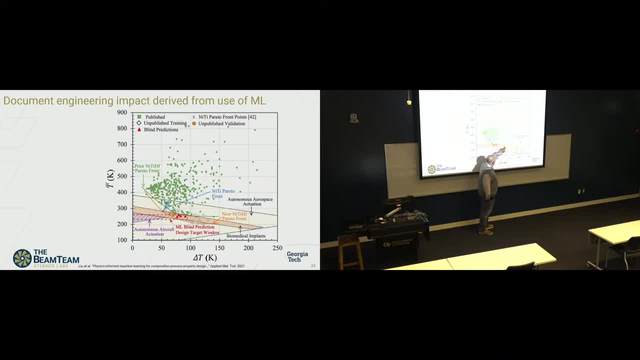 which is biomedical implants. It really opened up a whole new window in medical implants. Previously, stents and heart valves that we use out of nickel titanium are this little blue line on the edge- blue dot- And we opened up a whole new space of materials. 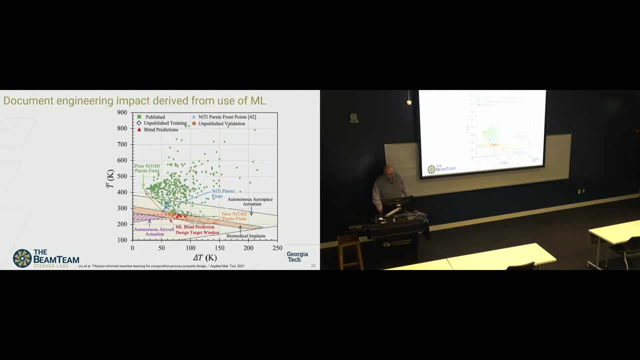 that we can use in a whole new range of medical implants with the work. So I think this documentation of what works and what doesn't work is really important and something engineers and domain scientists can do that computer scientists can't do with machine learning. 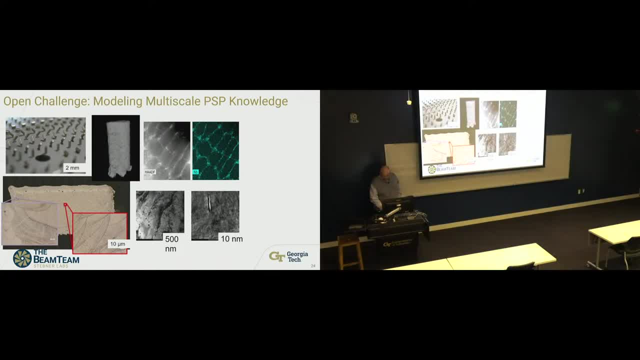 So I think that's an important thing too. All right, with all the technical difficulties, I'm gonna go a little fast, but where do I think some frontiers or grand challenges still are? I don't think we have machine learning that by itself today can understand like we as people can. 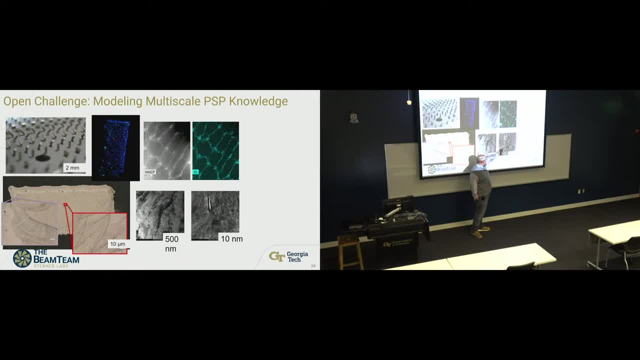 how atoms at the nanometer or sub-nanometer scale into defects at the mesoscale or microstructure features at the microscale right all the way up to the part scale at millimeters or meters, connect and create a process-structure property relationship. 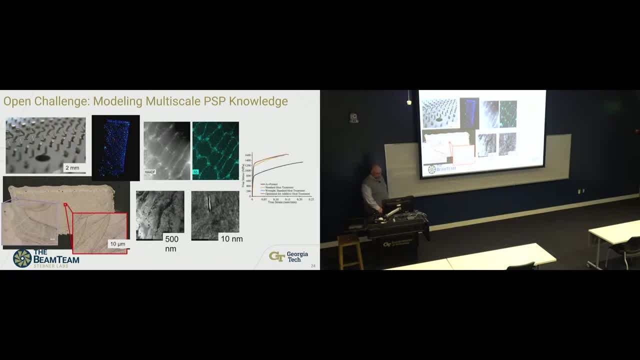 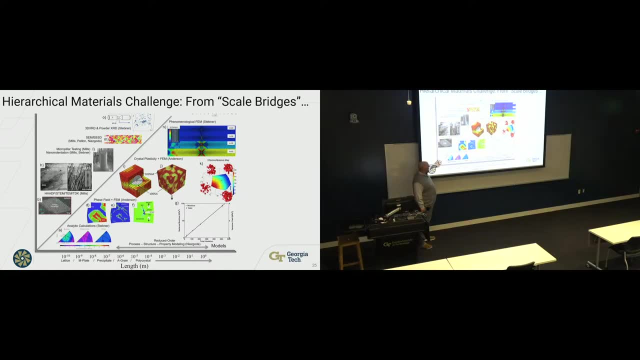 of a material in its application, And so I think that's one. you know the way I was brought up. you know the way I was brought up in graduate school was we were gonna do this through bridging scales, right? So being able to have models. 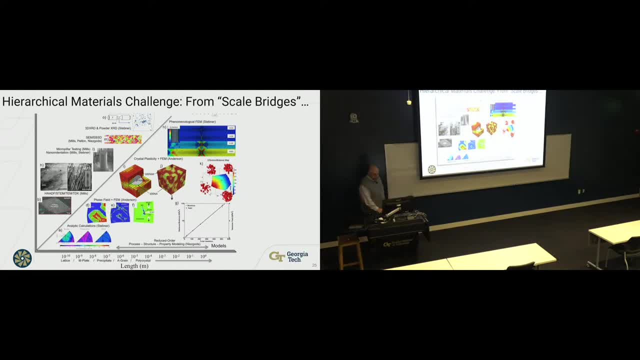 where we could either concurrently or hierarchically pass information from atoms up to meso, meso to micro, micro to macro. right. This was the pass from the physicist to the material scientist, all the way to the mechanical engineer. right was how we were gonna do this. 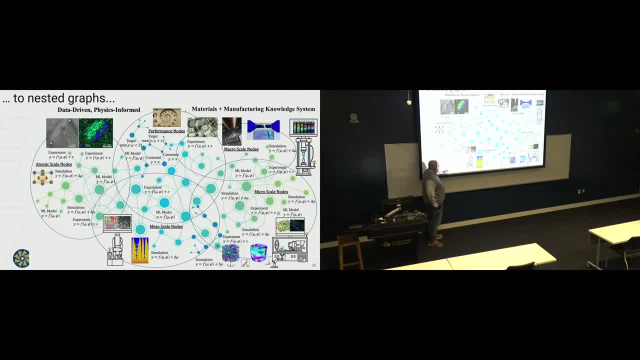 What we think about now in this data-driven world is: this is more a graph, where each ability to produce a piece of data, whether it's a DFT simulation, a phase field simulation, right, a mechanical test, whatever it is we're doing- 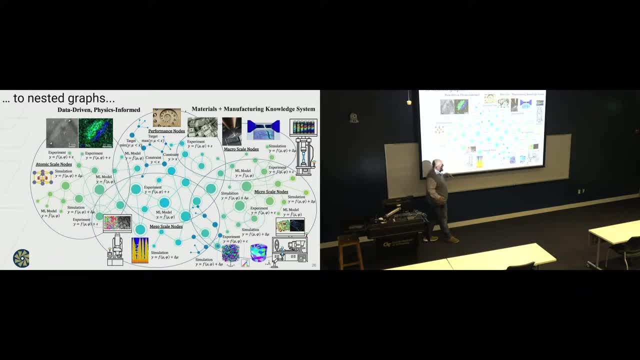 each data source becomes a node and then every time we wanna ask a question, we need a different collection of nodes to be connected to make a model to answer that question, And time and cost should factor into these nodes as well. right, and then behind each one of these. 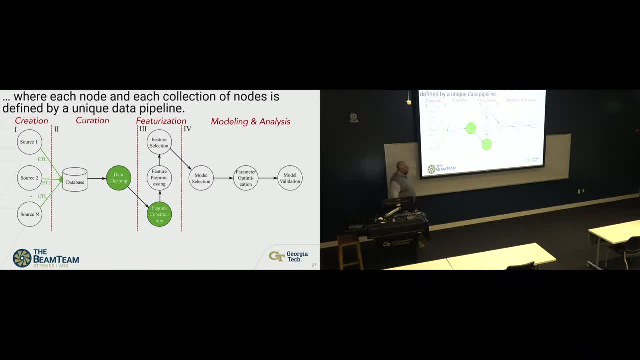 we get one of these pipelines right and we get a different model, And so I think the machine learning sits at the end there, and this is really where domain scientists can meet computer scientists and we can make advancements that they cannot. 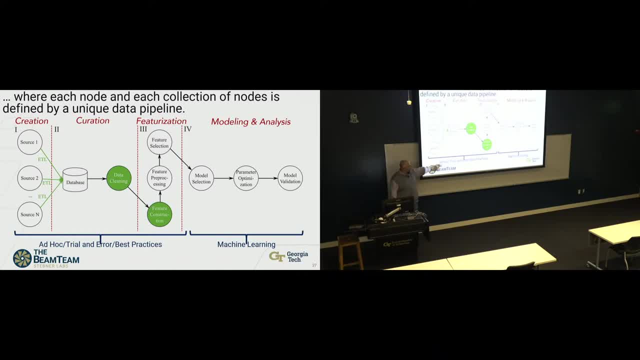 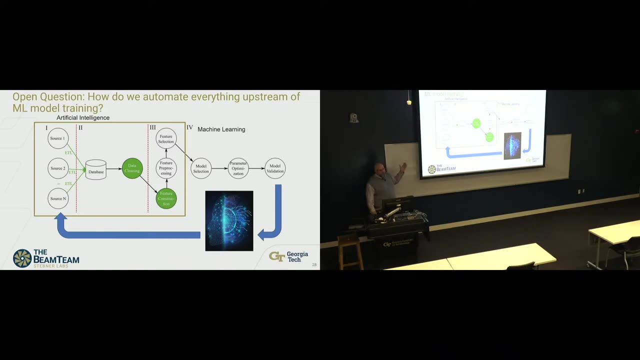 is, how do we get beyond these stages being done once for one data set and into general constructs and formats that work across multiple problems or multiple kinds of data, And so when we can really automate that, I think that's where we can really get into. 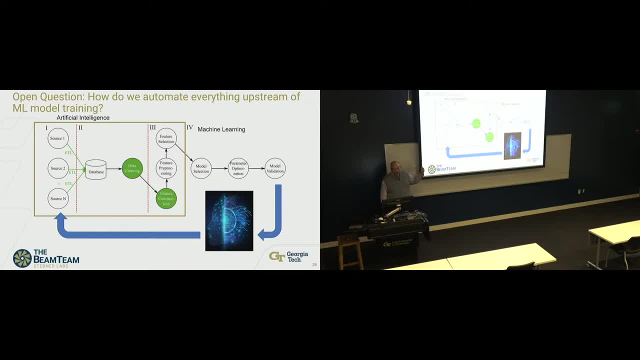 true AI assistance in our R&D or our commercialization efforts. right, So this is now. if we had automation for this piece, now, AI could actually interpret the uncertainty and results of the machine learning and suggest what data to create next. 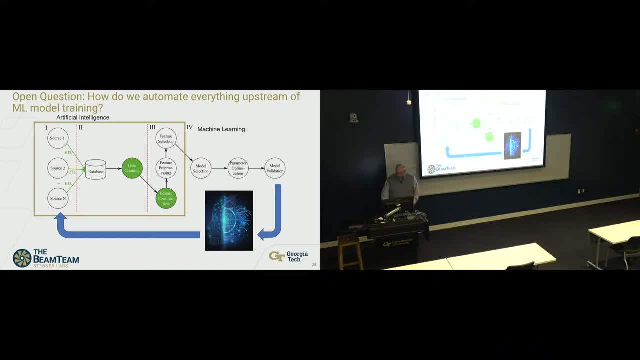 and it could automatically be processed and fed back into the model again. So there are some cases where this has been set up once or for a specific thing, like pharmaceutical development, but generally in the problems of materials to manufacturing there's not kind of general frameworks for these parts. 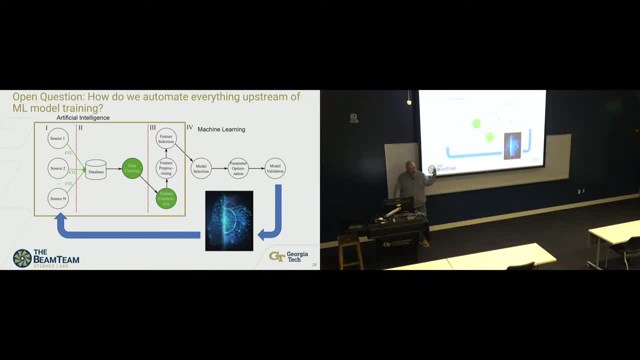 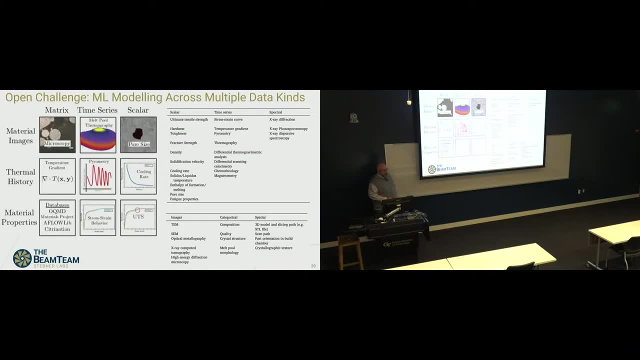 like. there are support: vector machines, Gaussian process models, neural networks, general machine learning constructs- for the last part, Okay- and then, of course, different kinds of data. So we need scalar data which are like yield strength, modulus time series data, the temperature profile. 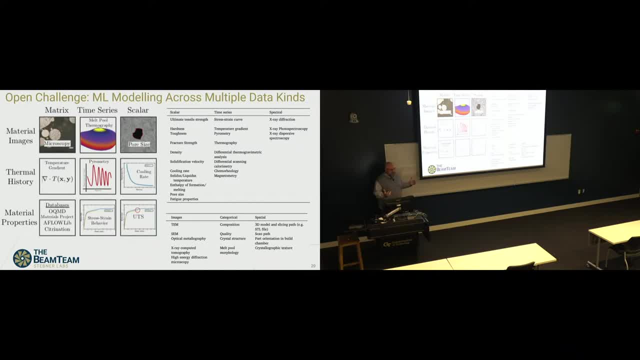 during the processing right Image data. we use images all over material science and manufacturing. We don't have machine learning right now where we can feed all these kinds of data and get one model fit to them all right, These large language models, ChatGPT. 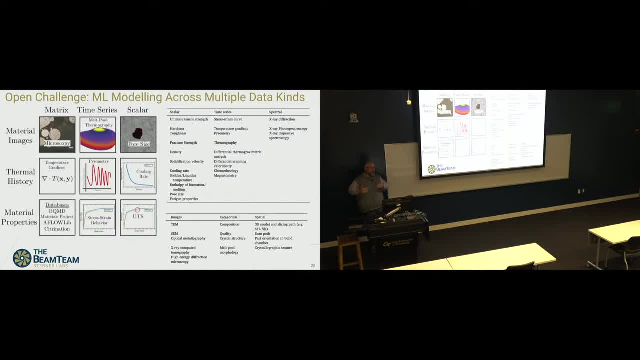 can kind of return to us a report that include these different types of data, but they still haven't made a model across all those kinds of data right. So we're trying to push there, but we haven't really gotten there yet. So I think this is a grand challenge we can work on. 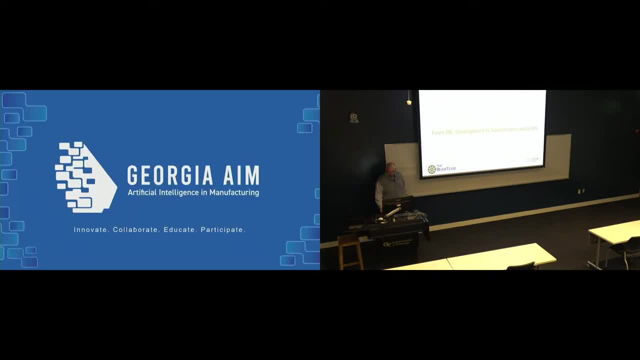 in all kinds of material science in manufacturing. Finally, with the last couple minutes I want to leave time For Q and A. we have a large effort being led out of Georgia Tech, but really spanning the whole state and the nation called Georgia AIM. 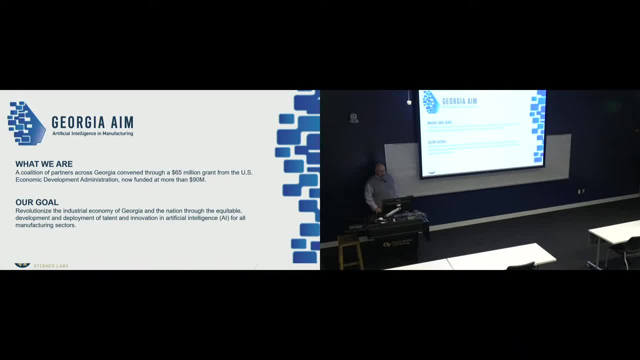 or Georgia, Artificial Intelligence and Manufacturing, And so we started with a $65 million investment from the Economic Development Agency. We've grown that portfolio quite a bit And we're really looking at equitable development and deployment of talent and innovation to enable artificial intelligence in all manufacturing sectors. 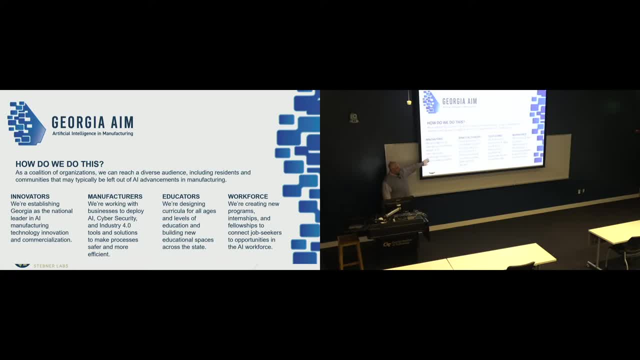 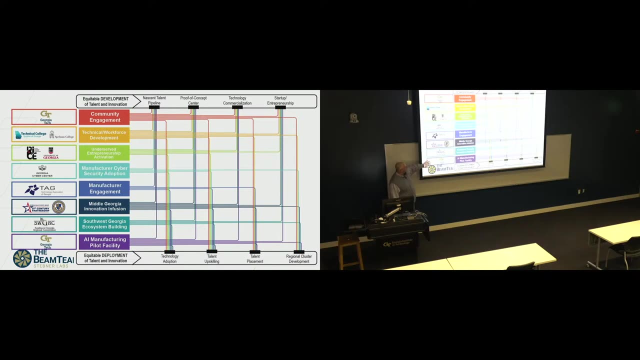 And so we have innovation or R&D programs, manufacturing programs, education programs and workforce training programs. We have a partnership- I don't know if I had the part- of more than 40 nonprofits, universities and colleges across the state that are enacting these through eight different programs. 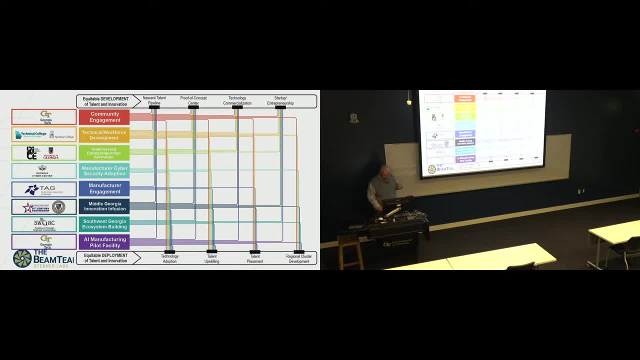 The bottom one here is our AI manufacturing pilot facility here at Georgia Tech. This is where I sit every day. It's just if you take just the diagonal, it's just a diagonal street that goes to Rocky Mountain Pizza, The end pill, all the way to the end where it hits 14th. 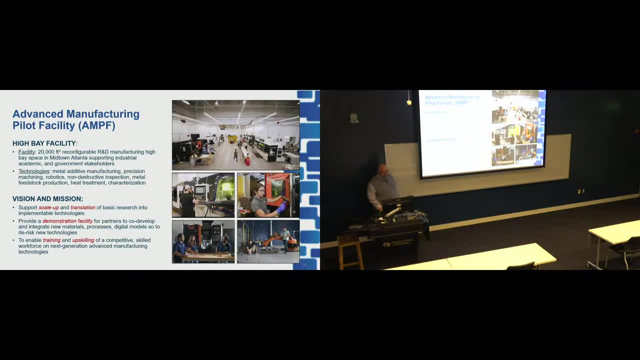 it's right on the corner there And it's a pretty cool facility. right now It's about a 20,000 square foot reconfigurable manufacturing and demonstration facility. So we have robotic machining, we have all kinds of metals, 3D printing. 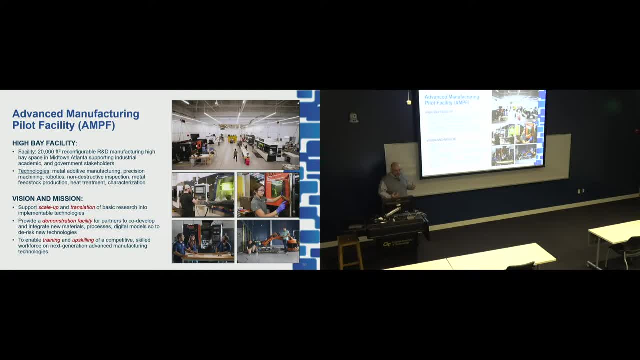 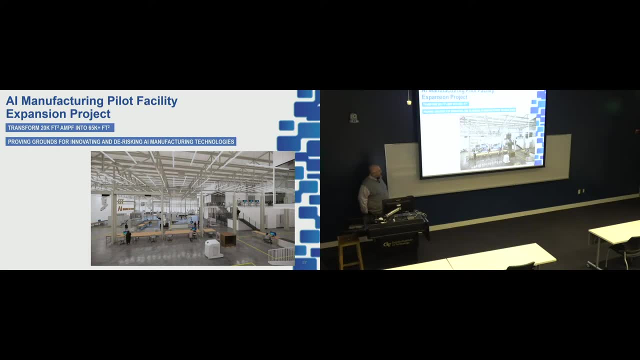 we can melt things, roll things, break things, look at their microstructures, right Heat, treat them, whatever- all these different kinds of things. But we're most exciting thing is this spring. actually demo starts end of this month. 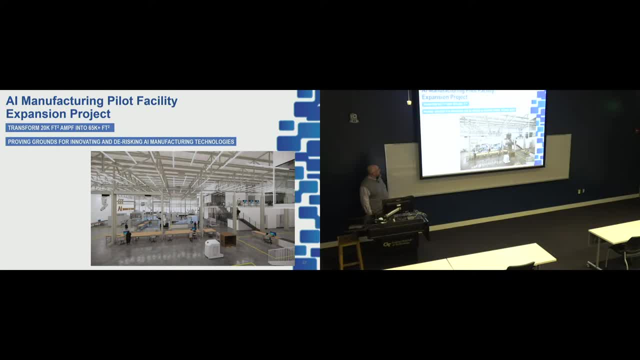 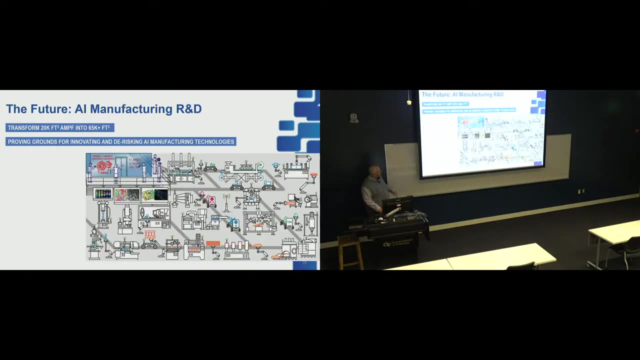 end of April We're gonna expand into a 65,000 square foot facility where it can be a proving grounds for innovating and de-risking AI manufacturing technologies, And so it'll open fully September of 2025.. And we're really connecting and automating. 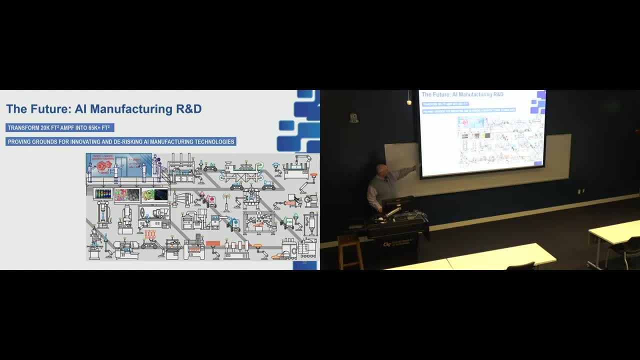 the ability to move samples from synthesis to recycling and everything in between- Semi-finished goods, test coupons, widgets- And we're also trying to put all the research tools to enable any researcher in any one of these domains that need to come together to enable AI. 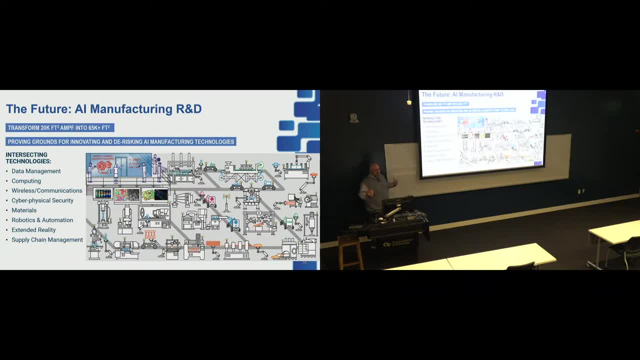 to be able to do their research there. So the whole thing's a user facility. Any student faculty at Georgia Tech can access it. Anyone in the nation can access it. We have people from national labs working there. We have companies with full-time employees there. 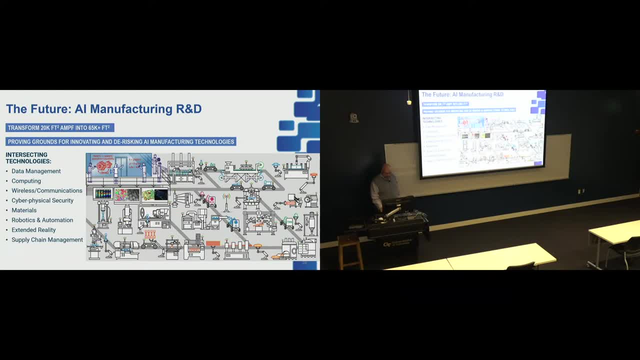 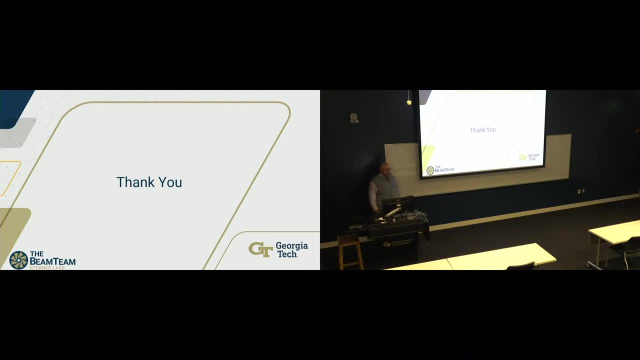 So it's a pretty neat facility where you can kind of innovate and come together, And if anybody's interested in more of that, let me know. I know some familiar faces but some new, But we have all kinds of opportunities there for undergraduates, graduate students, faculty alike. 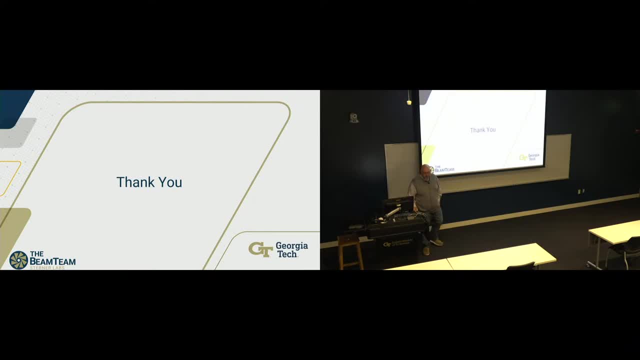 So feel free to contact me if you want to know more about that That. I'll thank you for your time. Time for a couple questions? Yeah, Sorry, Andre usually is loud. Thanks, I'm not loud enough, but we'll. 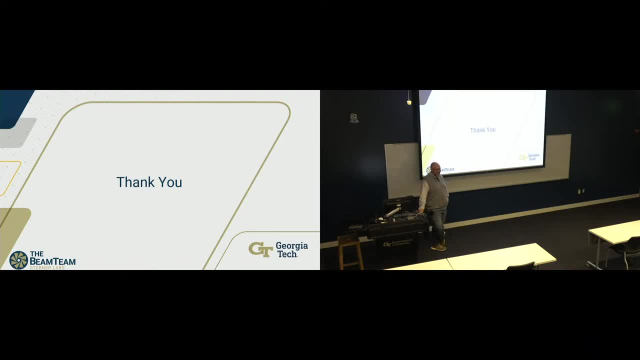 Yeah, but this is recorded. I learned that I have to be yeah speaking to Mike. So, Aaron, this is always wonderful how you lay out the whole logic of thinking, essentially for application scientists to get into a space of ML, statistical modeling, if you will. 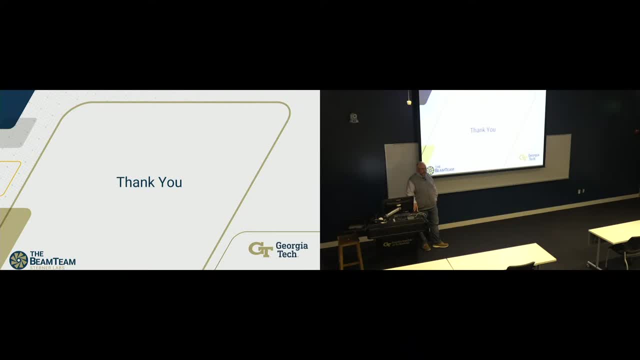 I am going to ask maybe a question more on your last part, when you outlined this open frontier, So you don't need to bring the slides. Sure, Mostly it's more of maybe it's a little philosophical or maybe it's not philosophical as it is. 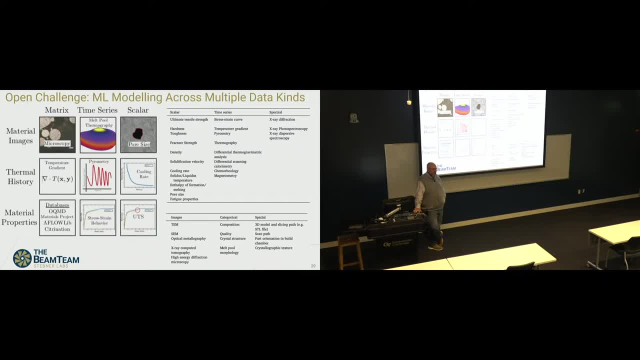 So the question is the following: When you outline all of these models- and they really can be categorical models or quantitative, but it's all collection of numbers and inputs, outputs, There could be constraint, noise, And even if it's a categorical model, 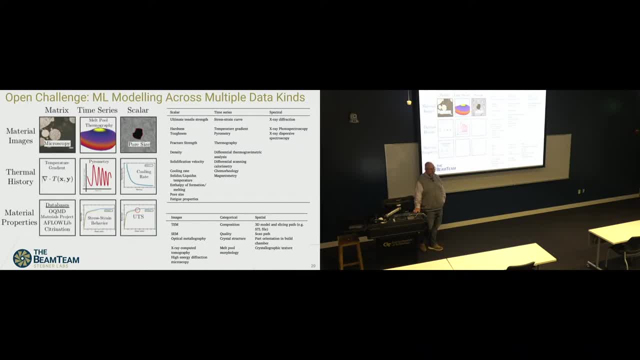 it's still numbers, right, It's one, two, three, so to speak. So the failure or the kind of the fundamental shortcut or the shortcomings of these types of models, since, even if they have inputs that are physics-based, 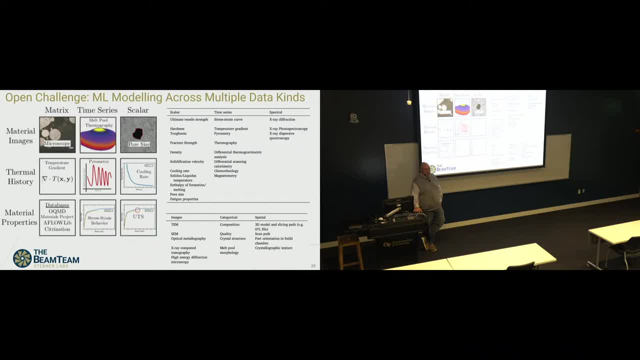 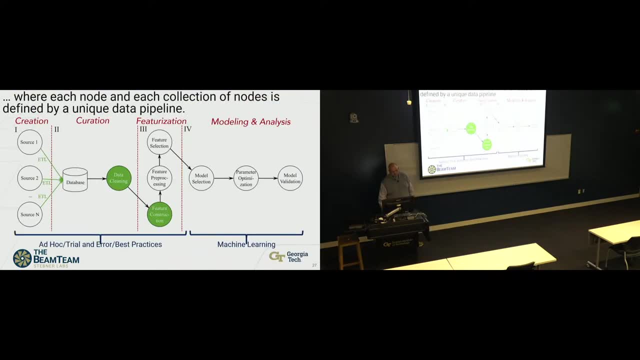 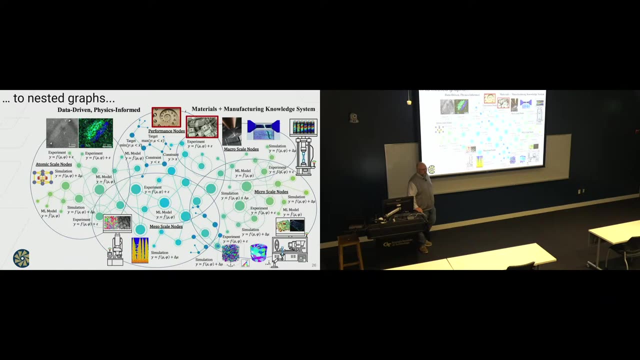 they do not really satisfy any laws right. So there's no such as energy conservation laws or mass conservation laws or momentum conservation laws, which is the critical piece: what engineering is? as far as validity, We do things, and that's our first check. 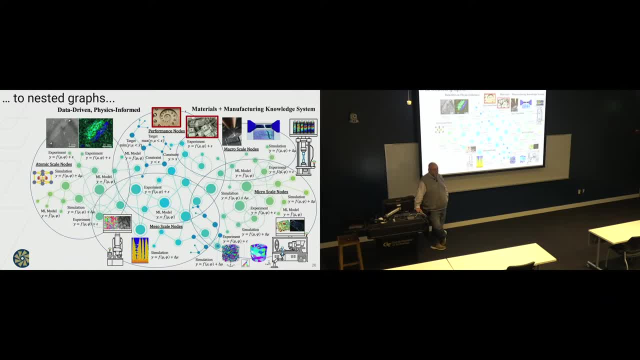 We don't want to violate these basic laws, And it's so easy to violate the basic laws with this model, Sure, So that's good. That's kind of my first question. Then, based on this, I'll build my second mini question. 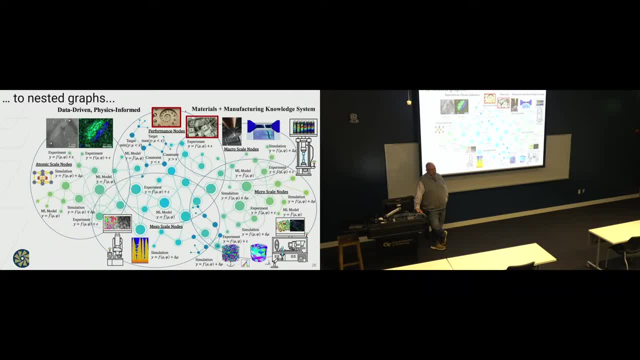 If you can comment on that. is that a fundamental flaw? It will be resolved. People are thinking about this. What's the deal there? Yeah, it's another one of the pitfalls that many engineers fall into when they first think they can just feed their data into some Python library. 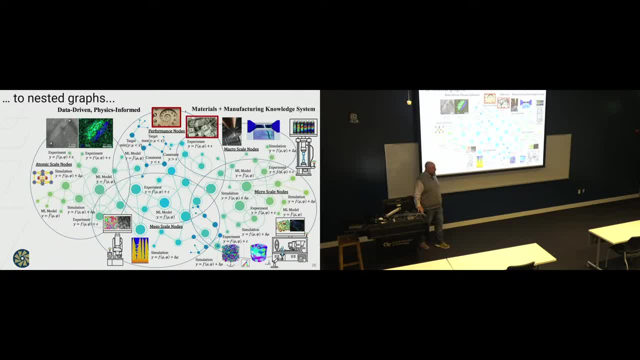 and use the answer right away without any further thought. right, And so I think the way we treat this is those, You know, physics-based models, which are called simulations. in this picture we rewrite those like the machine learning model, but recognizing the uncertainty is in the assumptions. 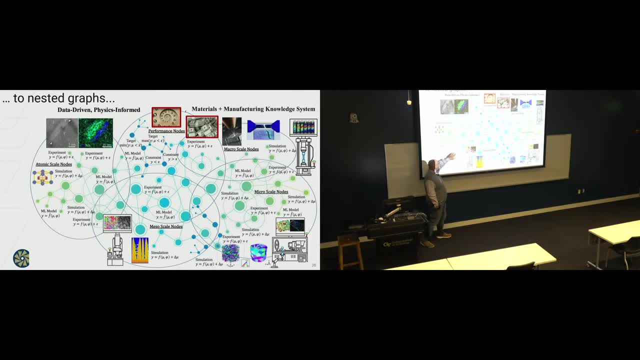 from all the physics into only the ones we put in the model where the machine learning, the uncertainty, is in that functional form. We don't have all those laws cooked in to the functional form or the basis functions, But we can actually put these together. 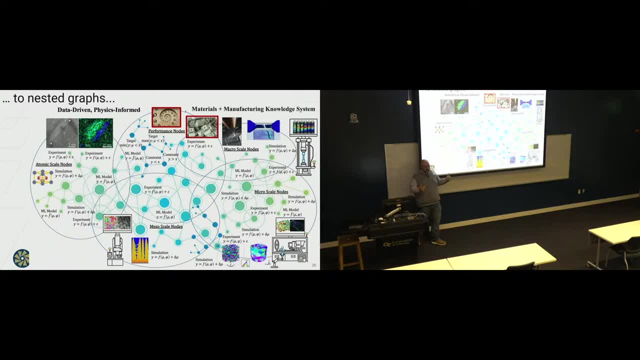 And in fact, one of the things we're doing for invertible models now is forcing those functional forms for the machine learning to be the ODM, ODEs or PDEs of the physics that we use to describe the physics A. so we know that they are continuously differentiable. 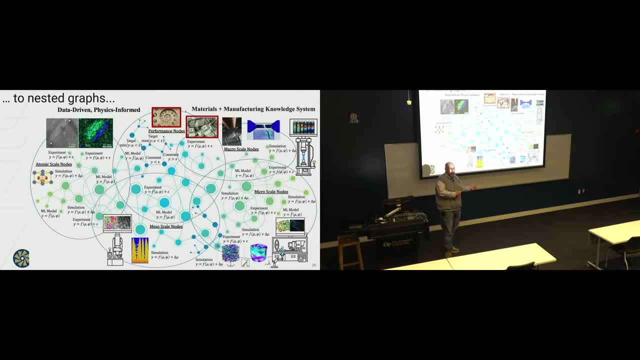 and we can invert them. They're guaranteed to be invertible when we wanna use them. But B then we can put the same constraints on them as we would. the physics-based model and our UQ of the machine learning model that fits different weights and functional forms. 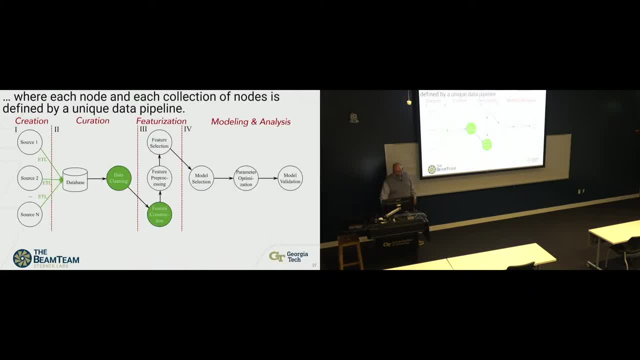 to the PDEs themselves. So I think that's really where one of these opportunities and feature construction. this is not only the features of the data, but this can be the features of the basis functions that we put into the machine learning as well. 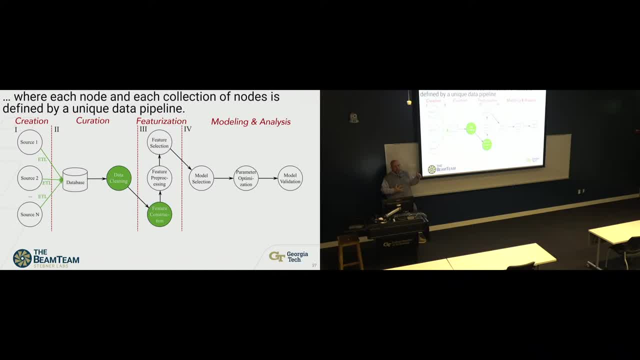 And that's that opportunity to combine the physics knowledge, domain expertise and hundreds of years of learning in with these statistical approaches right, And to bake them in there. Yeah, that's great. So maybe that's my second mini question- kind of falls into right into this domain. 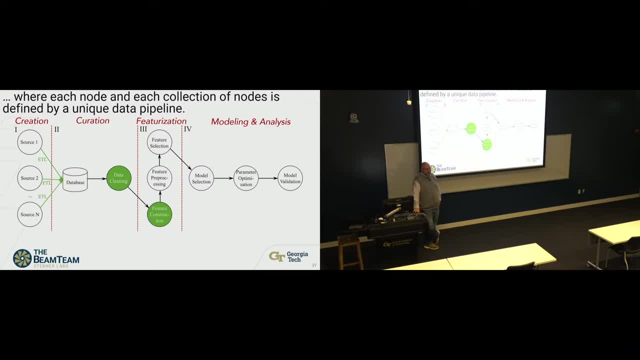 So it feels like what would be extremely powerful if, instead of the inputs and outputs being a bunch of datas, organized in some sort of multidimensional space, whatever the vectors, and even if it's a differentiable, and so on, if you look at the challenge of chat GPTs, 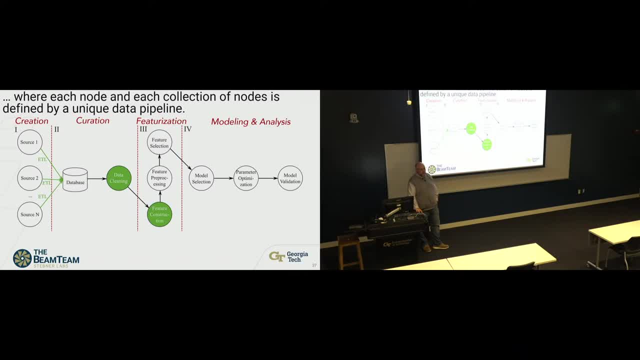 any generation right To me. that's where you look. the amount of compute that needs to go to produce a, so to speak, reasoning of four-year-old child And the scaling is obviously non-trivial, wrong, essentially, In essence, any meaningful intelligence. quote unquote. 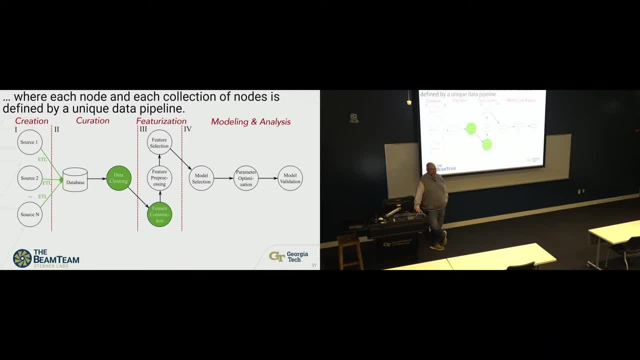 whatever you define is out of reach with current approaches. So my question now in the domain of engineering, so much of the physical description, let's say how the fluid flows in very complex geometries we actually describe very reliably using differential equations. 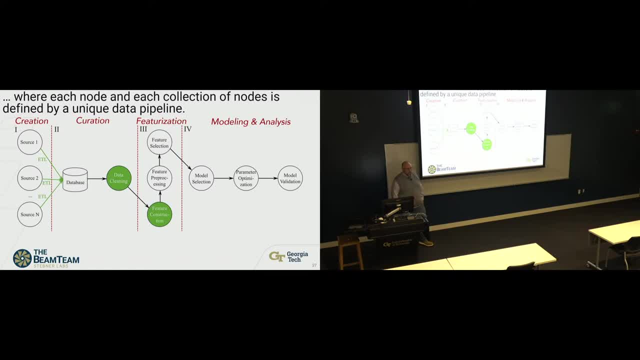 Like, let's say, Navier-Stokes equation. It works, it's satisfied the laws. Can the models, AI models, ML models- be created using the equations as inputs? So no data, no conversion, everything is done on the. so these are construct and you build around this. 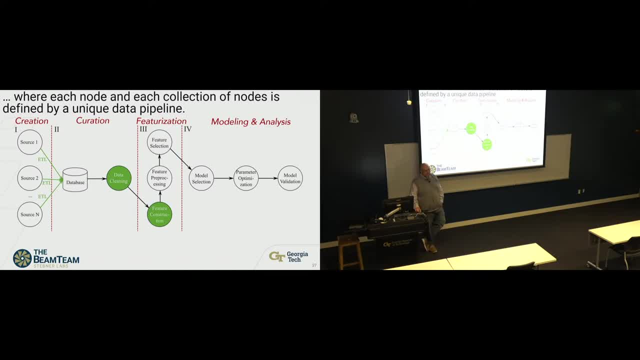 And so- and the goal is really here is not only fundamentally satisfies basic laws, but also, like what you're trying to do right now, but also hopefully it will bring the penalty or cost of this simulation down to meaningful numbers. Yeah, So there's two ways that that is being done. 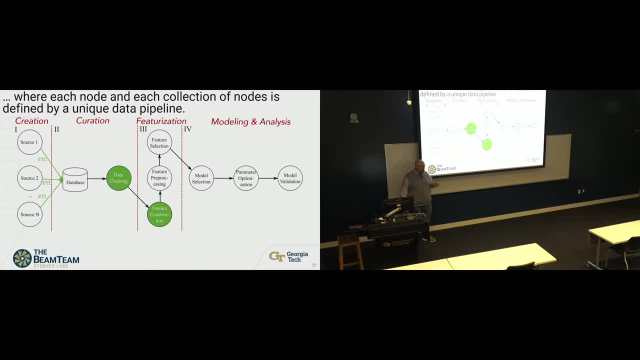 One is to build you're probably really familiar with is the surrogate modeling, right? So actually building a statistical model of the differential equation, right, But that's a little unsatisfying for the reasons you mentioned at the start. We had a really good speaker actually. 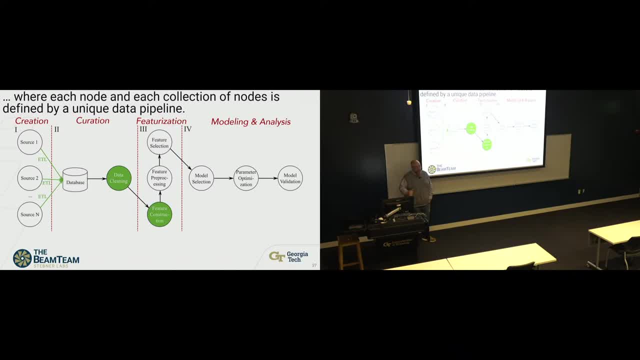 in the mechanics series- earlier Kaushik Bhattacharya from Caltech, where they're actually using the ODEs as the basis functions or activation functions in neural networks, so that you are naturally baking the constitutive model in and now you're just tuning the model parameters. 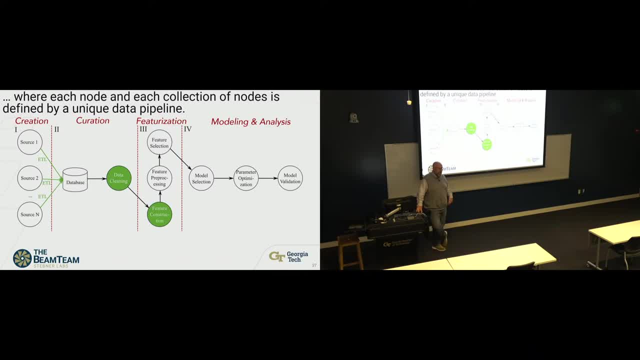 to your data right using the machine learning methods, And so I think this process of physics informed or physics constrained constitutive modeling is something that's happening, and there's really a lot of exciting work. Unfortunately, my own work- I've been driven away from constitutive modeling. 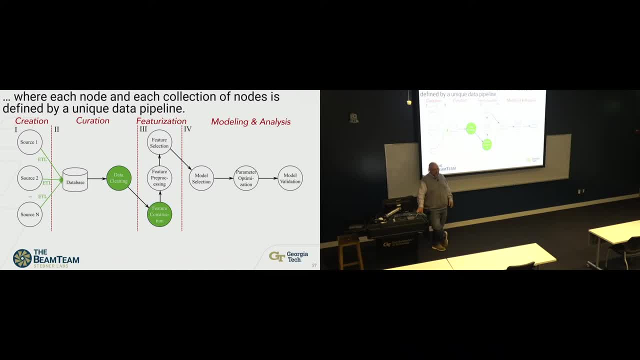 for all the manufacturing and automation stuff for the last five years, but I've been following the field a bit and I still think it's a really cool area And I think it's one of these places where engineers and scientists can innovate in data science. 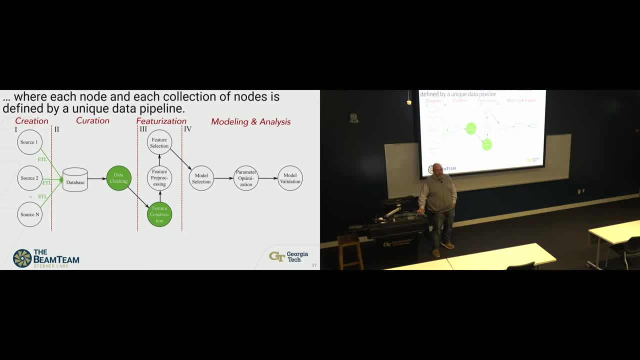 where computer scientists, for the most part, will not right. So I think, yeah, it's a pretty good area. Maybe one more question? Sure, Yeah, it's very interesting. Andre took my first question, so I have a second question. 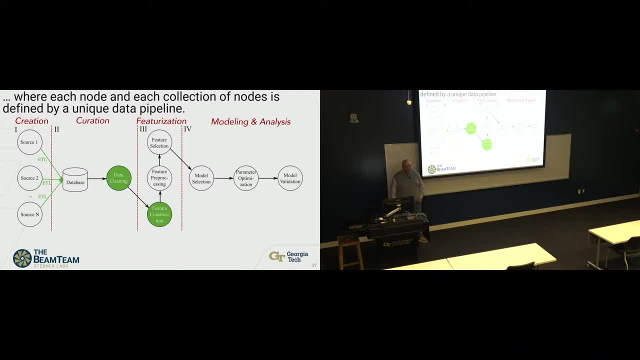 Yeah, So you know I work in electronic materials. One of the challenges in electronic materials is that the properties are impacted by things that you can't really measure right. So the whole part. that's why we have a clean room, right. 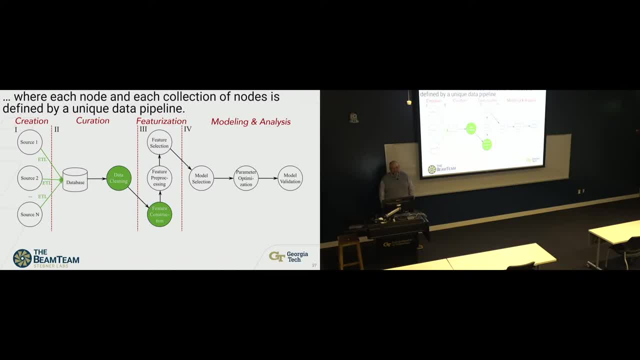 Part per million, part per billion? You can't measure the structure. How do you envision if that's the case, where you have key variables that literally you can't measure? is there a way to inform the ML model what those may be? 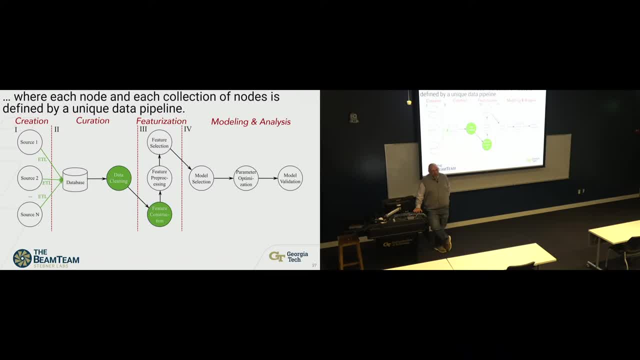 or how do you handle something like that? Yeah, so I actually worked on one of these problems for CoorsTek back when I was at School of Mines. So there's a similar thing in abnormal grain growth in ceramics- right Where the abnormal grain growth bound is often triggered. 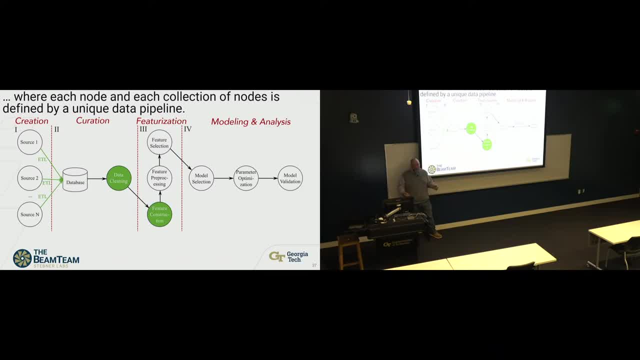 by parts per billion of a silicon defect or magnesium element in there or something like that. Very similar problem, just with a different scale and structural materials in mind. right, And that gets back to my thing: Machine learning isn't the magic solution for everything. 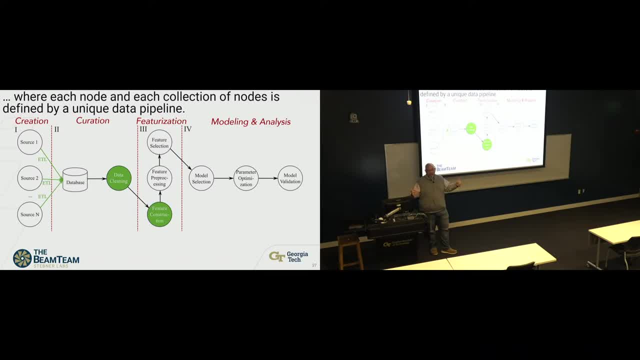 and it can't magically know something that doesn't exist in the data right. And so I think that there are. so where we've looked and where we got inspired, like that maximum defect problem where again the company was most concerned about that extreme outlier. 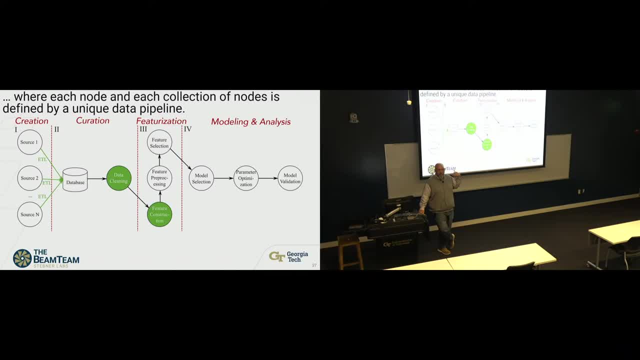 that happened once out of every 2,000 parts, not the one that was happening in every part, right is? there are similar theories in weather prediction, so hurricane prediction, that kind of stuff, and it actually dates back to the mining industry. 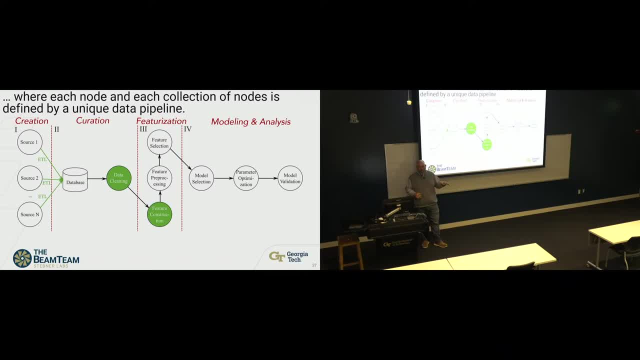 The theories are actually called nugget theories, where it was like: how do I find the nugget of gold, given all this massive expanse right, And how do you do this? I guess my answer is: we can do it about as well as we can predict hurricanes or predict the weather right. 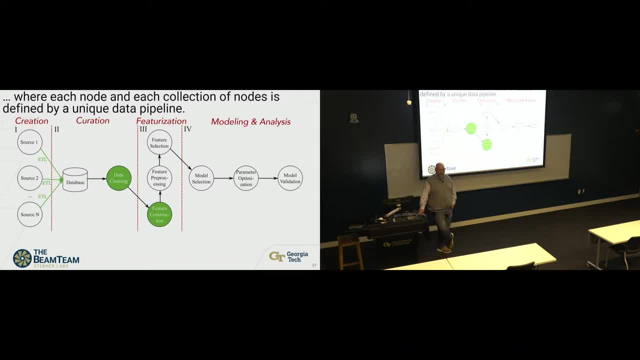 And so you can get it right a lot of days, but sometimes you miss a big one Right, And so, at least based on my current experience with it- but I do think this is another frontier of research- I think some of the things that are working very well. 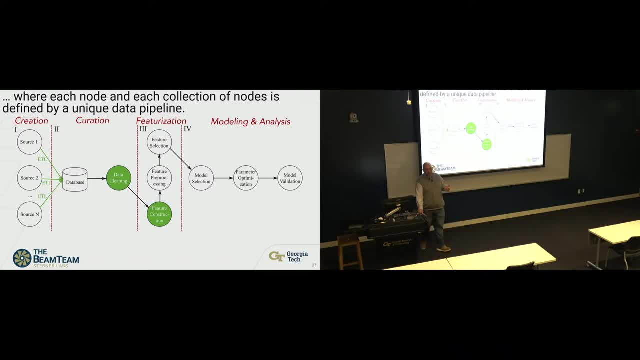 are in the fields of treating it as an anomaly, detection or a change in process, Like maybe I can't measure that one thing, but can I measure its effect and know that the process has changed and then correlate it to whatever might have happened in that moment? right, 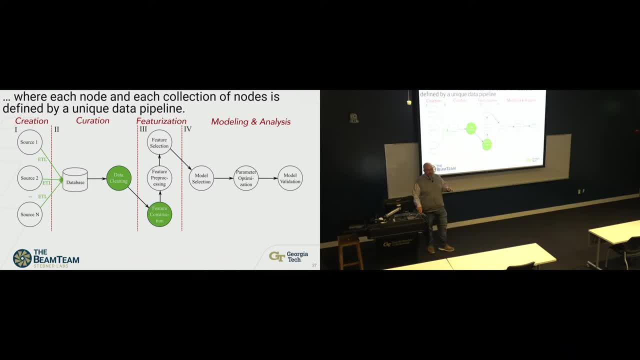 And so if it's really that difficult to predict, it's not going to happen. And so if you, if it's really that difficult to predict, it's not going to happen, And so if it's really that difficult to measure, or that expense, you know. 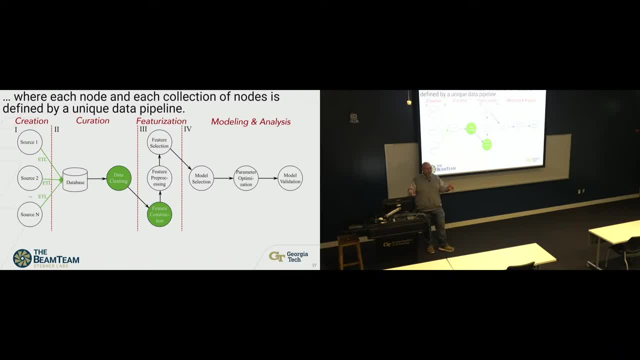 something like a part per billion defect. now you got to do whatever. it is time of flight sims and there's five instruments in the you know five hour vicinity where you can do that and you can get on them once a month or whatever, right. 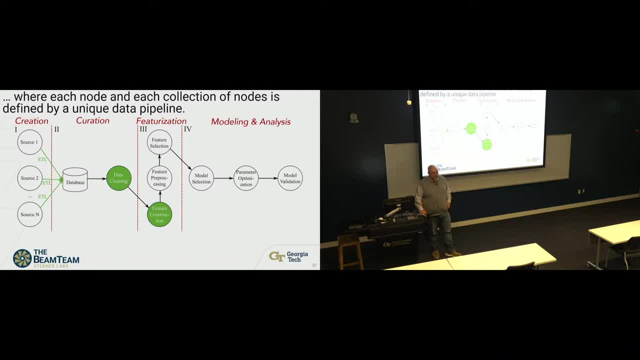 We have similar things with synchrotron work we do right. Maybe you can do that expensive one where you can observe it and correlate it to all the things you can measure in the lab and now have that indirect model of it that works in the laboratory or in your process, right?